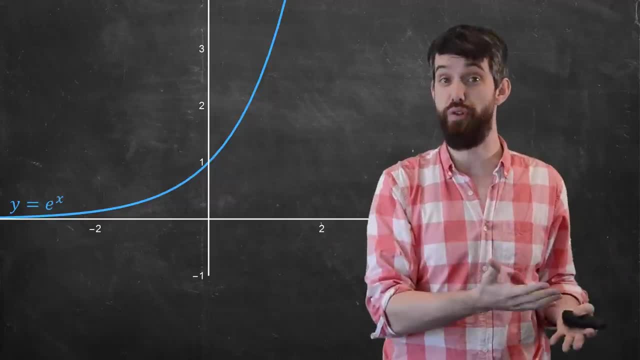 you could do is say: look, e to the 0 is a number that you know, e to the 0 is just 1.. Well, that's not going to help you. You're going to have to figure out. well, what is. 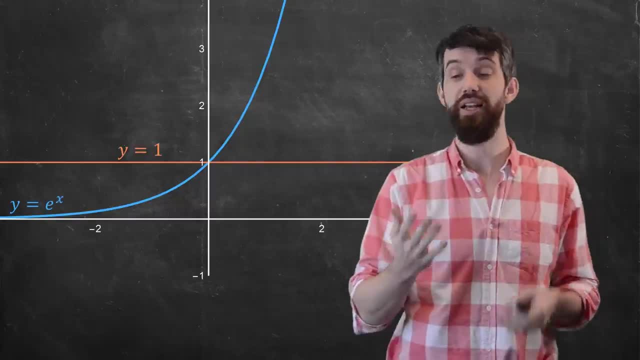 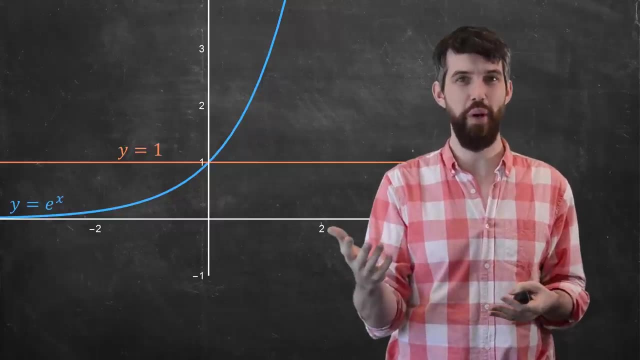 e to the 0?. So what if I considered, instead of e to the x, just y equal to 1, the constant function 1?? Now, approximating e to the 0.2 by 1, it's not bad, There's a sort of like. 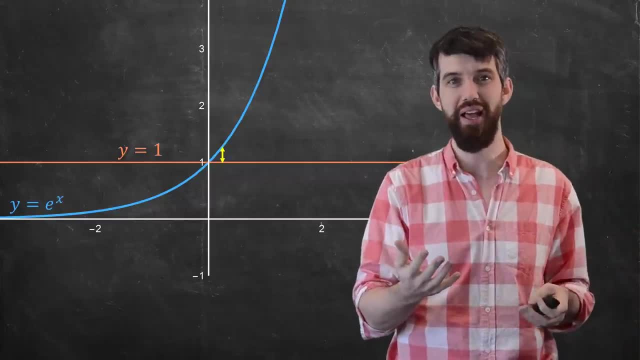 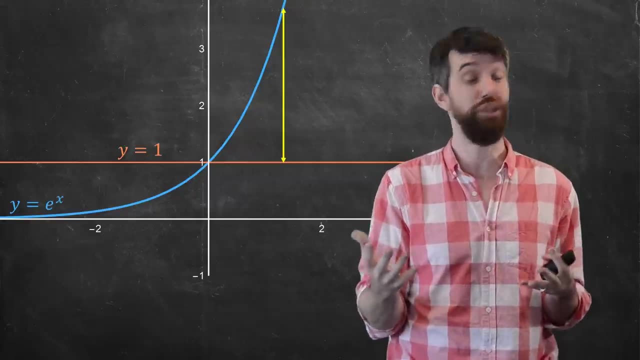 little error that remains here. It's not that gross of an error. But if I considered e somewhere larger and further away from 0, well, this error grows to be really, really large. and it grows to be large pretty quickly. But in calculus we developed a better way to figure. 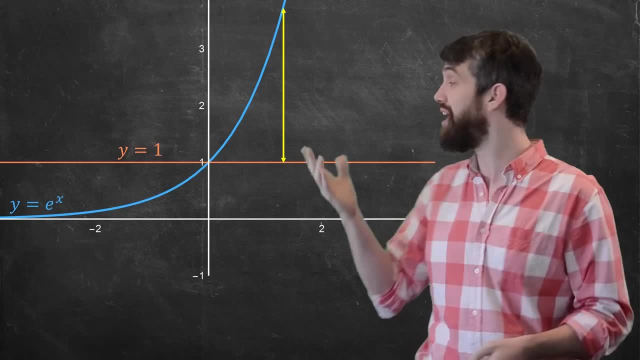 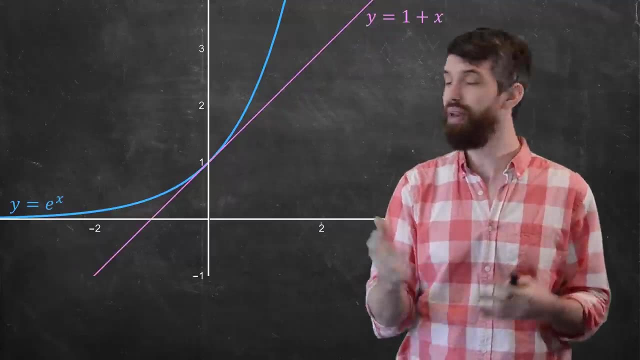 out how to do this. We had the idea of a linear approximation. So instead of a constant function, a constant line, what we're going to do instead is have a tangent line. Now, for this tangent line, our approximations are actually quite a bit better. It is a better. 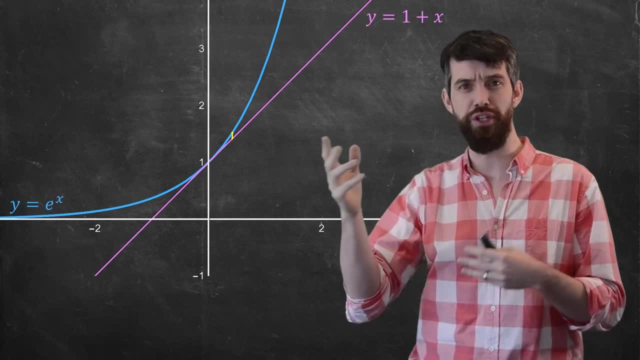 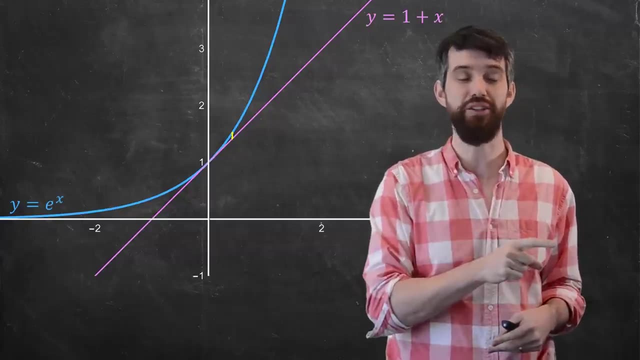 approximation, And the closer that you go to wherever you've put the tangent line- in this case it's the tangent line at 0,- the better your approximation gets. So this tangent line is pretty good, But can we do better than that? Can we do? 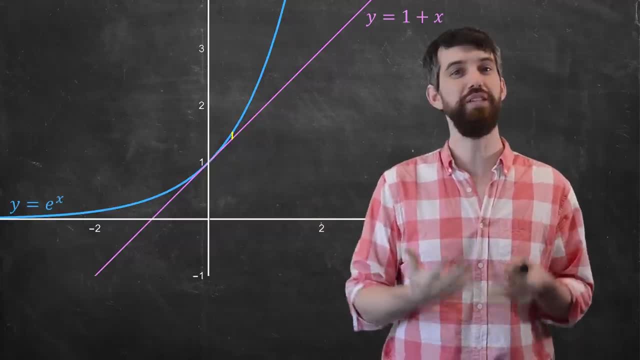 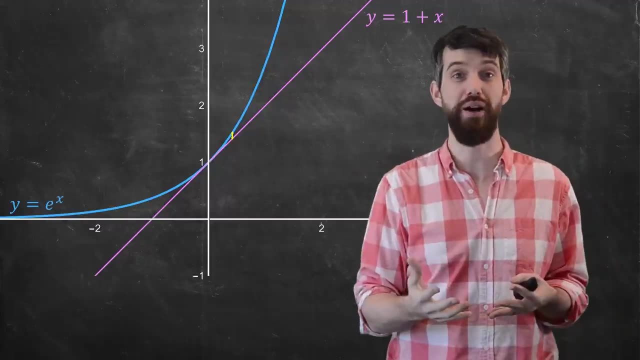 better than just a linear approximation. For example, imagine I instead try to put a quadratic, not a line, a quadratic as the thing that was going to approximate e to the x around the value of x equal to 0. Maybe it would look a little bit like this one. 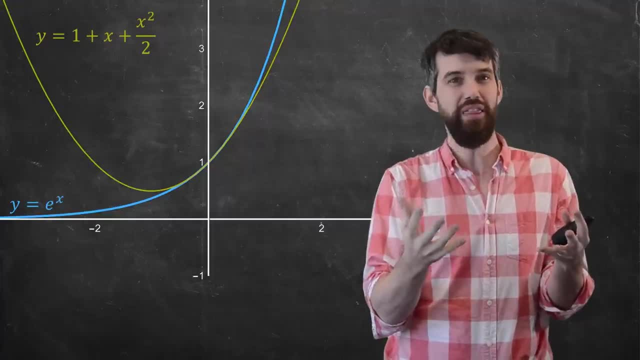 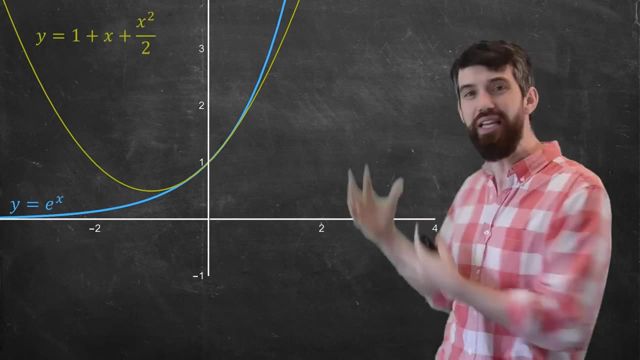 where I curl it up and I put in a quadratic, and I make the quadratic just touch at the point of x, equal to 0, and have a very similar slope and it just really nicely aligns. And now my error is actually pretty good. 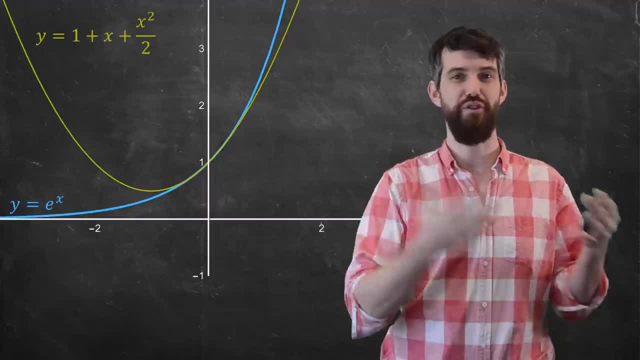 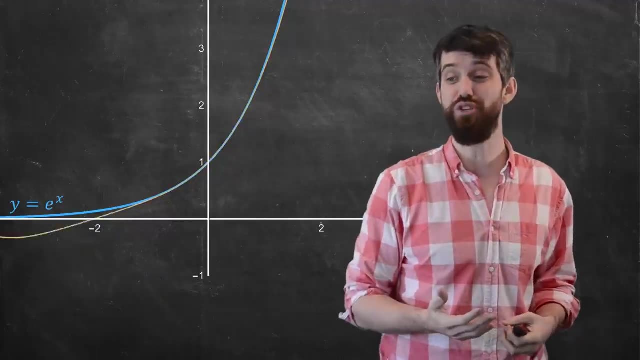 There's almost no space that I can visualize at all, And if I can do that for a quadratic, I can do the same kind of things for a cubic. It becomes an even better approximation, And I can even go further to a quartic or however long you want, to do as many turns as you. 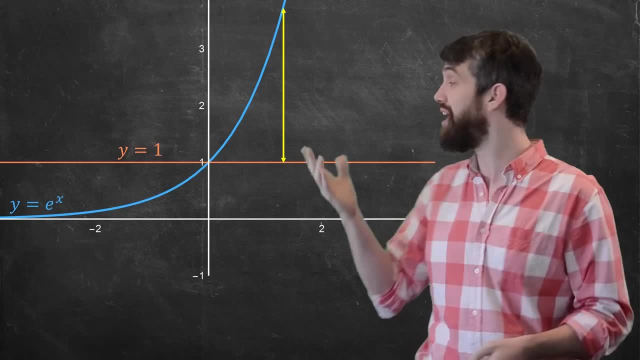 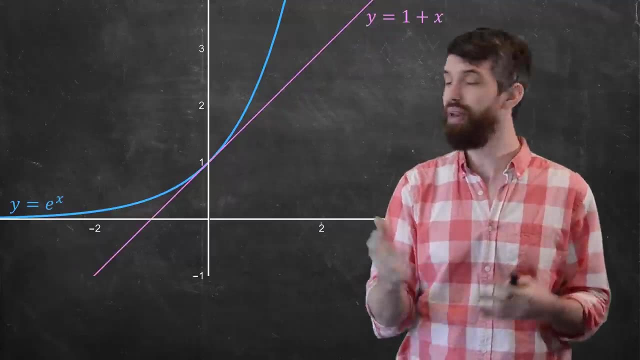 out how to do this. We had the idea of a linear approximation. So instead of a constant function, a constant line, what we're going to do instead is have a tangent line. Now, for this tangent line, our approximations are actually quite a bit better. It is a better. 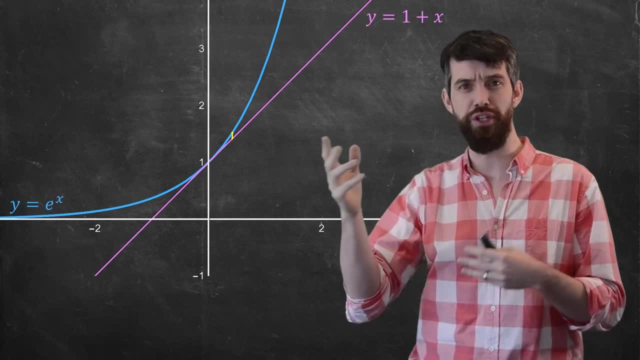 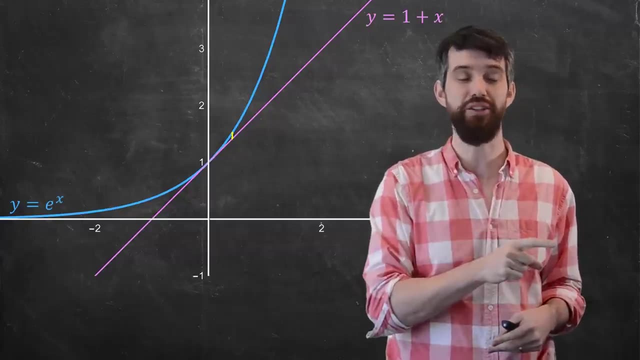 approximation, And the closer that you go to wherever you've put the tangent line- in this case it's the tangent line at 0,- the better your approximation gets. So this tangent line is pretty good, But can we do better than that? Can we do? 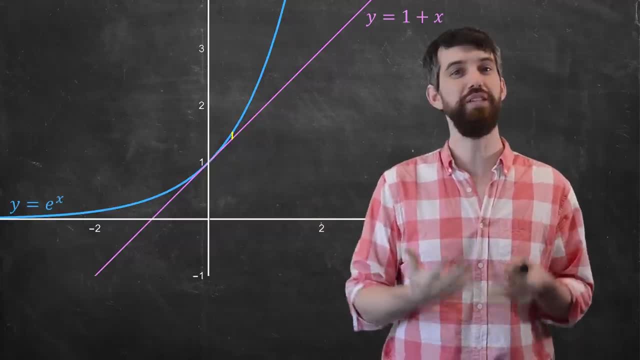 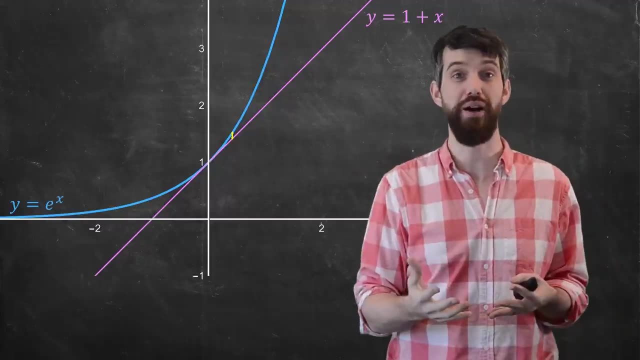 better than just a linear approximation. For example, imagine I instead try to put a quadratic, not a line, a quadratic as the thing that was going to approximate e to the x around the value of x equal to 0. Maybe it would look a little bit like this one. 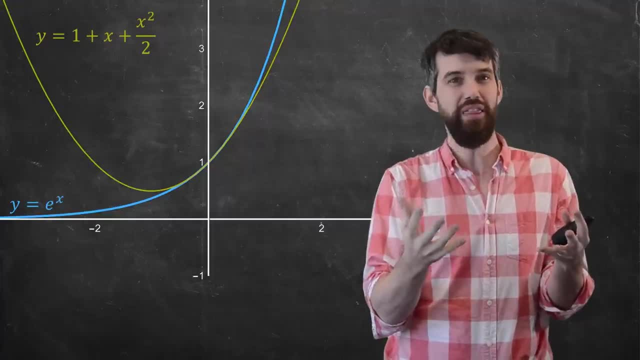 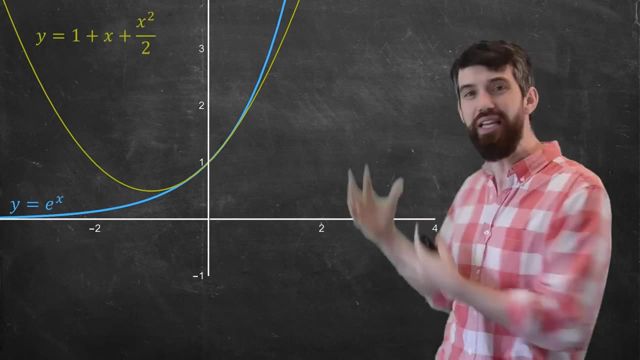 where I curl it up and I put in a quadratic, and I make the quadratic just touch at the point of x, equal to 0, and to have a very similar slope, and it just really nicely aligns. And now my error is actually pretty good. 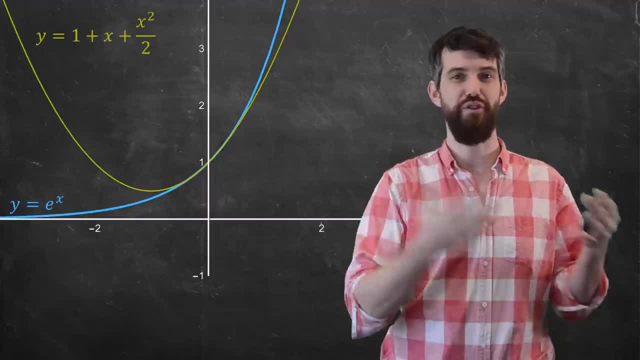 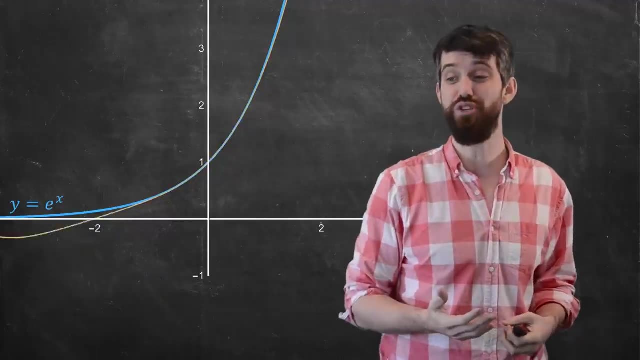 There's almost no space that I can visualize at all, And if I can do that for a quadratic, I can do the same kind of things for a cubic. It becomes an even better approximation, And I can even go further to a quartic or however long you want, to do as many turns as you. 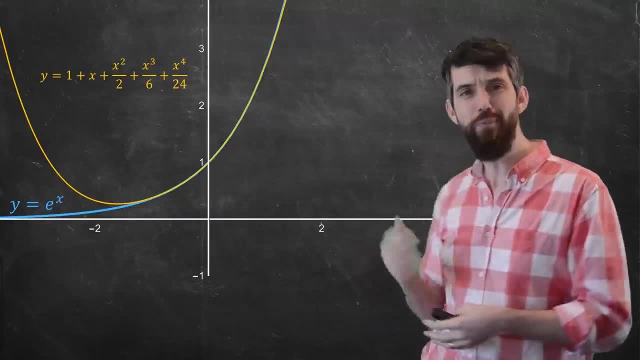 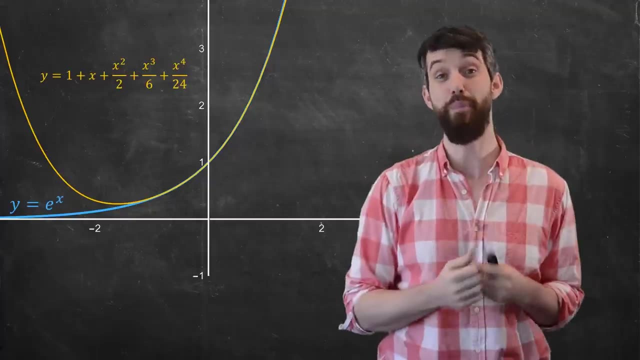 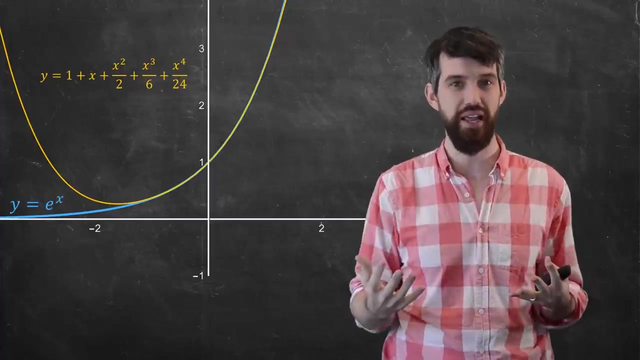 might wish. But how do I come up with these polynomials that so nicely approximate in some little region? How do I know whether this is the best a polynomial to approximate with And how good of an approximation really is it? And that is going to be the core of our study of Taylor series. And then, if I want to put 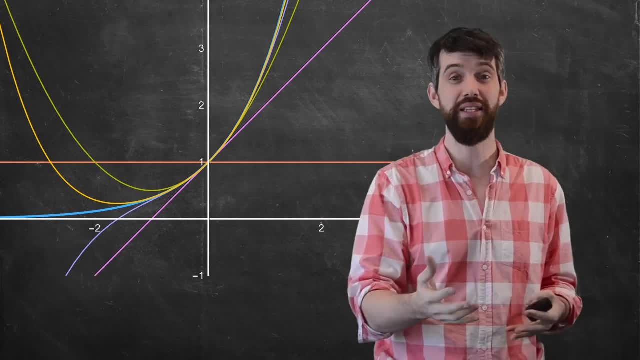 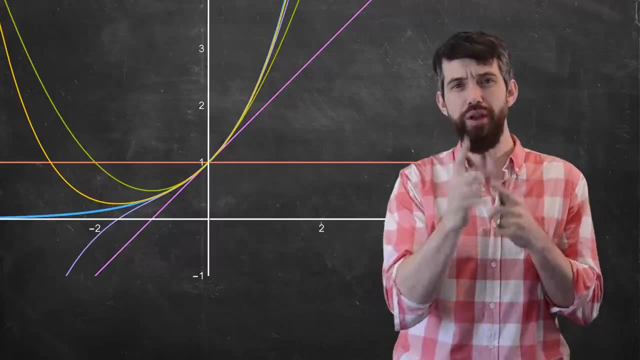 all of these on top of each other. I have the blue e to the x and I put the constant, the linear, the quadratic, the cubic and the quartic approximations all on the screen And what you can see is that the higher the degree of the polynomial, for example the 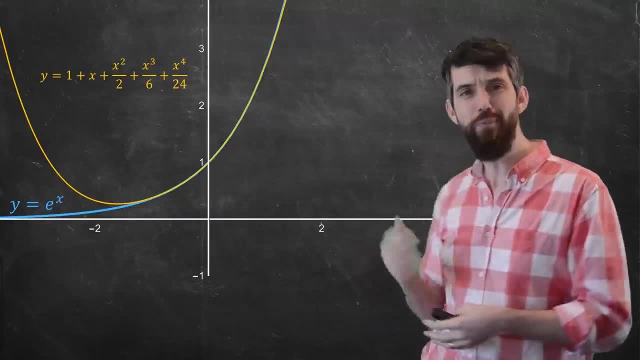 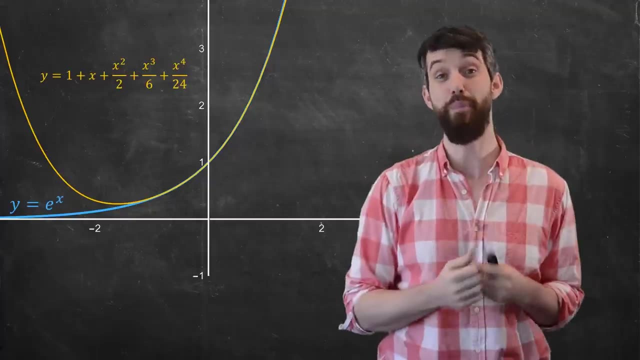 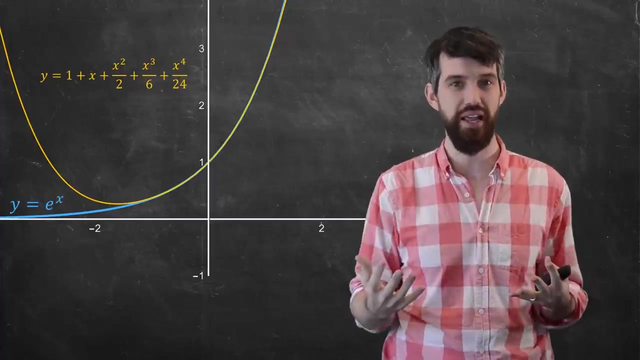 might wish. But how do I come up with these polynomials that so nicely approximate in some little region? How do I know whether this is the best a polynomial to approximate with And how good of an approximation really is it? And that is going to be the core of our study of Taylor series. And then, if I want to put 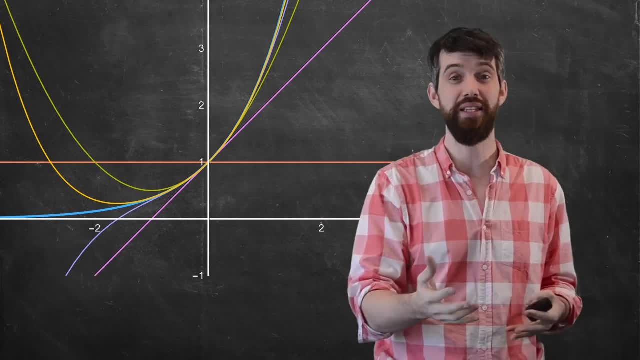 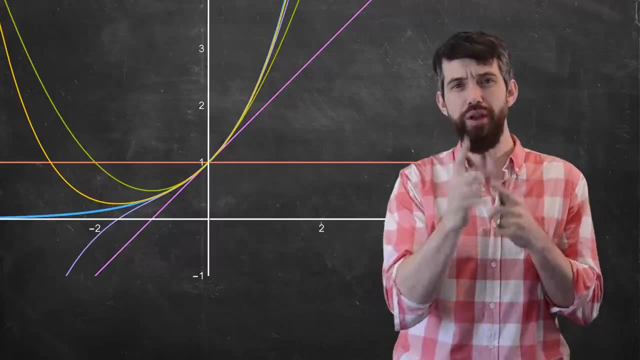 all of these on top of each other. I have the blue e to the x and I put the constant, the linear, the quadratic, the cubic and the quartic approximations all on the screen And what you can see is that the higher the degree of the polynomial, for example the 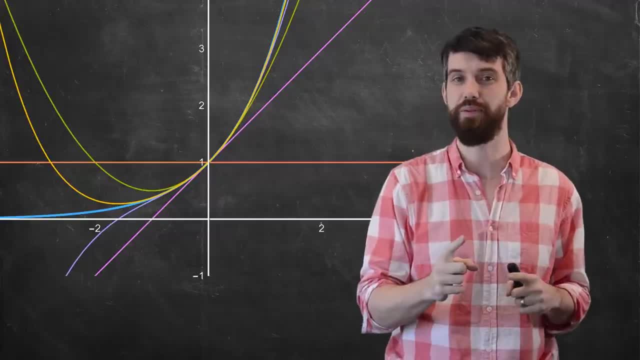 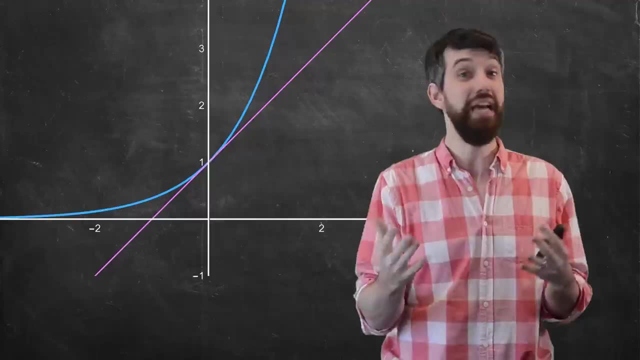 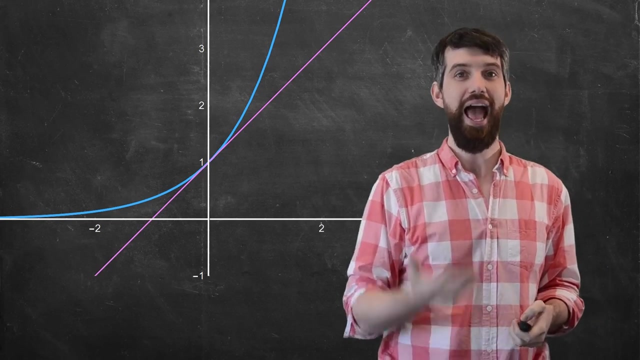 quartic, the better the approximation becomes. Alright. so let's go all the way back to linearization when we just approximated with the tangent line, So what I did there, and then we're going to generalize. So the first thing we say that when I'm doing a tangent line is that at the value of x equal. 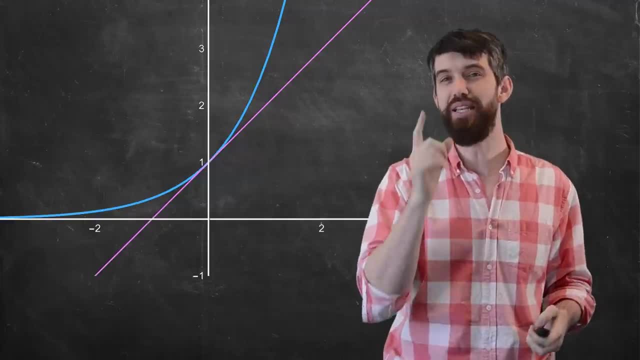 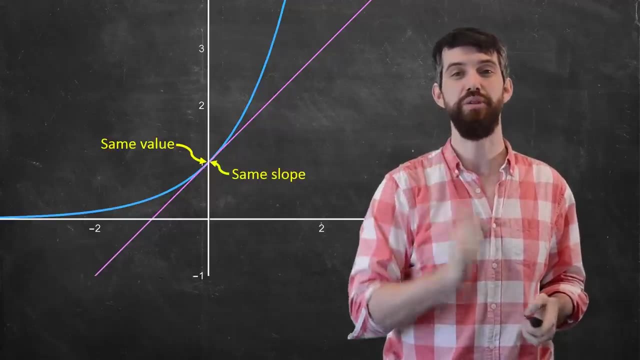 to 0,, the spot where my tangent line is at. I'm saying that the function and the tangent line have the same actual value, their y's are the same, but also they have the same slope. So those are my two different considerations. 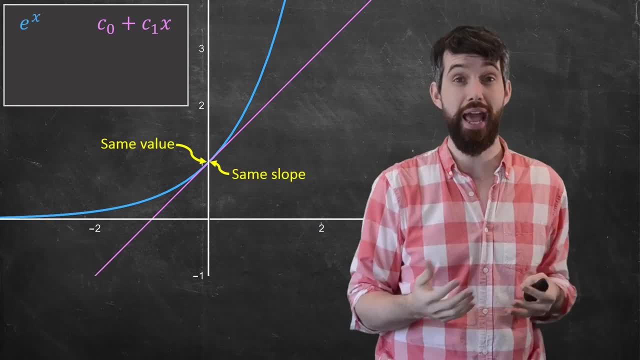 So, for example, if I compare e to the x, the function that I have and a generic linear, a generic linear of the form c0 plus c1x. That's what I'm going to do. So I'm going to do a tangent line and then I'm going to 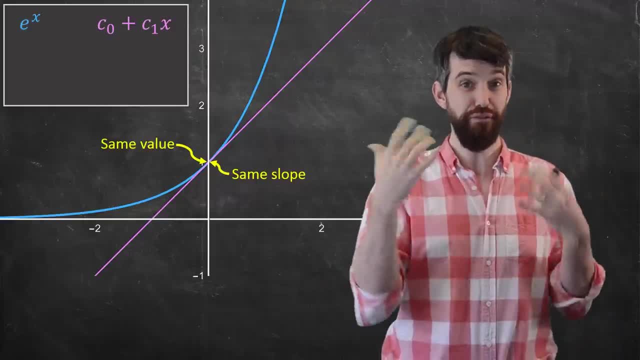 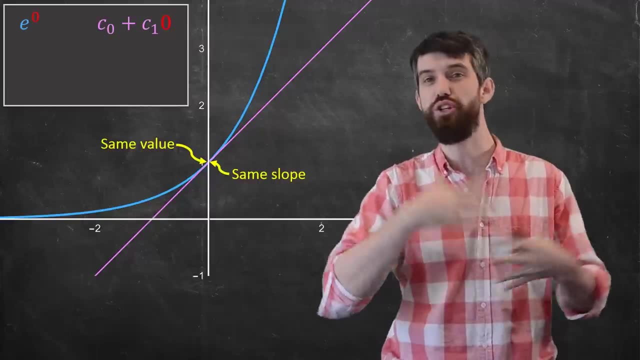 say that's what I mean by a completely generic linear function, Then the first thing I want to do is say that at the value of x equal to 0, they're exactly equal, So I can plug in x equal to 0.. e to the 0 is 1, c1 times 0 would be 0. 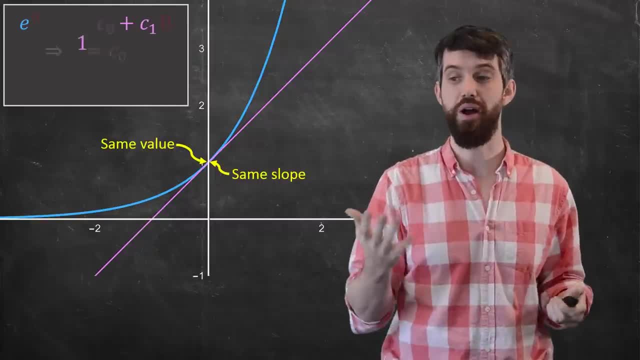 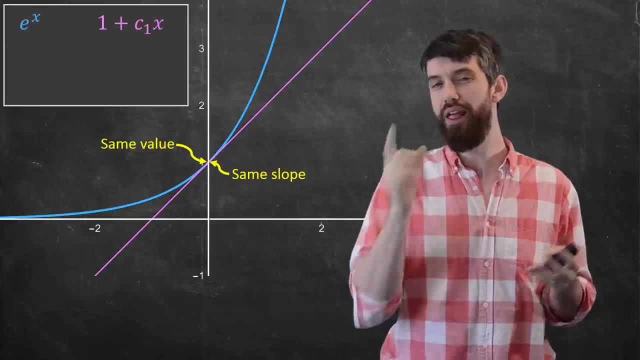 That just leaves me with c0 being 1.. Okay, not so bad, so I can put that in. Now I've got 1 plus some constant times, x and e to the x is what I'm going to compare, But then what I'm going to do is take the slopes being equal. 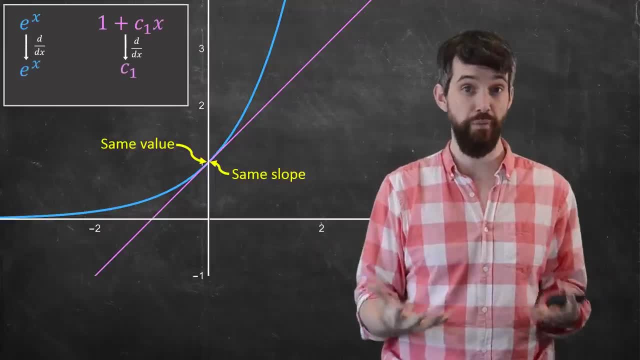 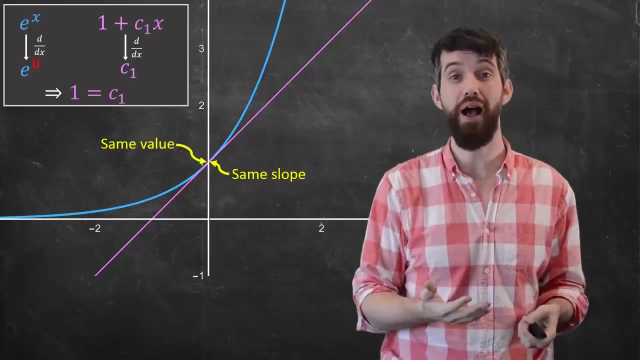 Now the slopes mean: take the derivative. So I'll take the derivative of both, and then, if I plug 0 into that, e to the 0 is again 1, and I get that our c1 is 1 as well. So what do we have? 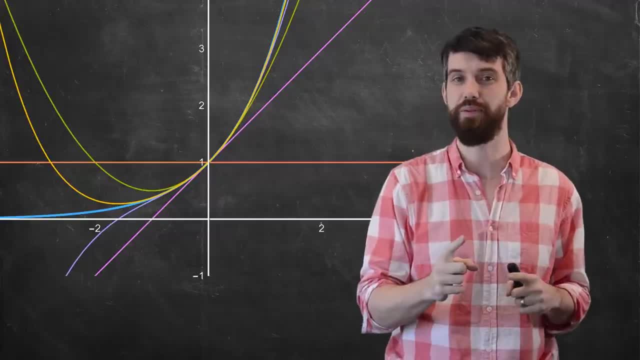 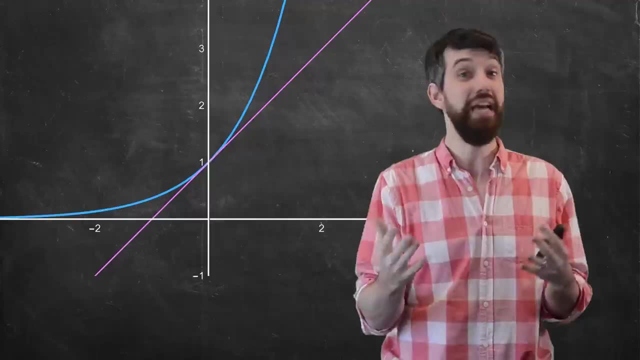 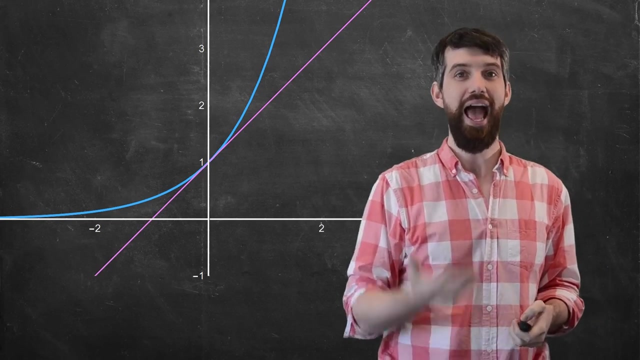 quartic, the better the approximation becomes All right. so let's go all the way back to linearization when we just approximated with the tangent line What I did there and then we're going to generalize. So the first thing we say that when I'm doing a tangent line is that at the value of x equal. 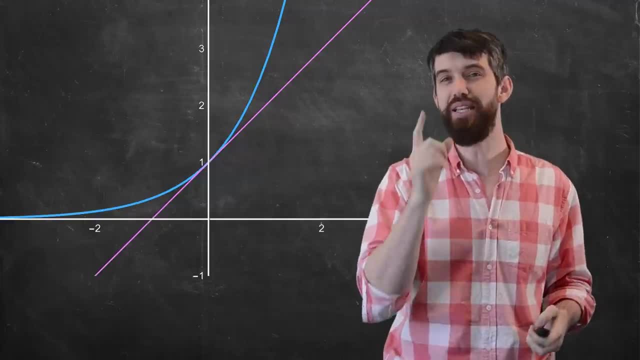 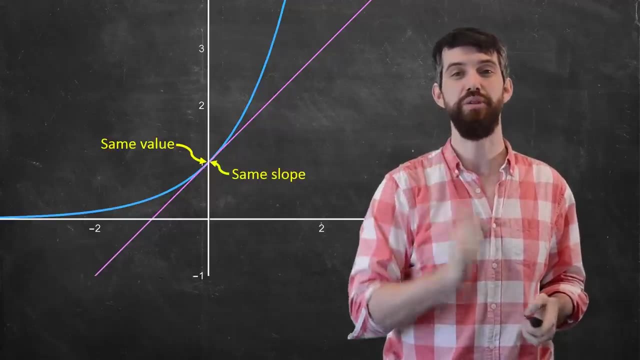 to 0,, the spot where my tangent line is at. I'm saying that the function and the tangent line have the same actual value, their y's are the same, but also they have the same slope. So those are my two different considerations. 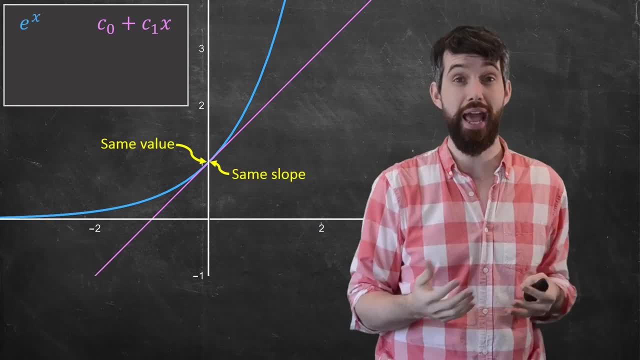 So, for example, if I compare e to the x, the function that I have and a generic linear, a generic linear of the form c0 plus c1x. That's what I'm going to do. So I'm going to do a tangent line and then I'm going to 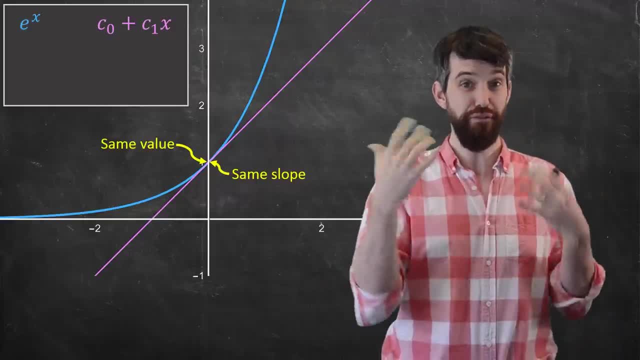 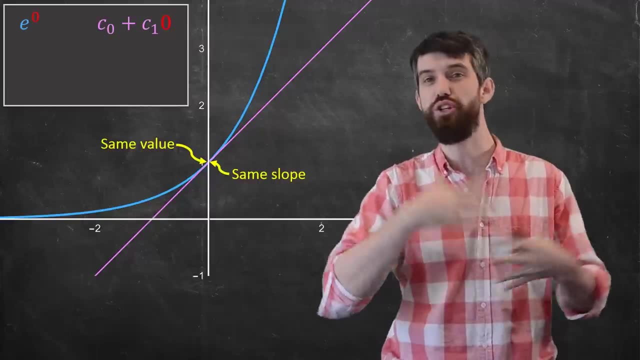 say that's what I mean by a completely generic linear function, Then the first thing I want to do is say that at the value of x equal to 0, they're exactly equal, So I can plug in x equal to 0.. e to the 0 is 1, c1 times 0 would be 0. 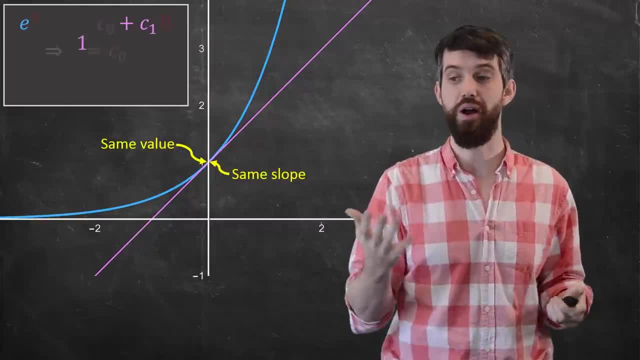 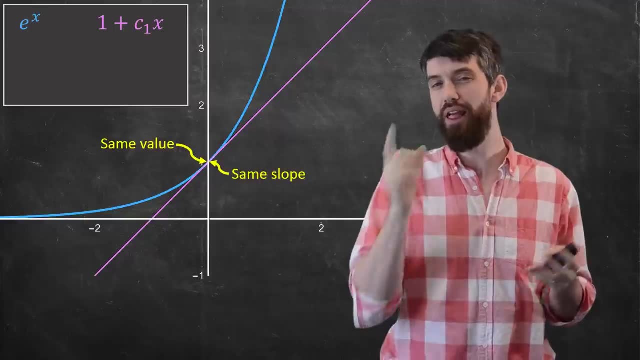 That just leaves me with c0 being 1.. Okay, not so bad, so I can put that in. Now I've got 1 plus some constant times, x and e to the x. these are what I can compare, But then what I'm going to do is take the slopes being equal. now, the slopes mean take. 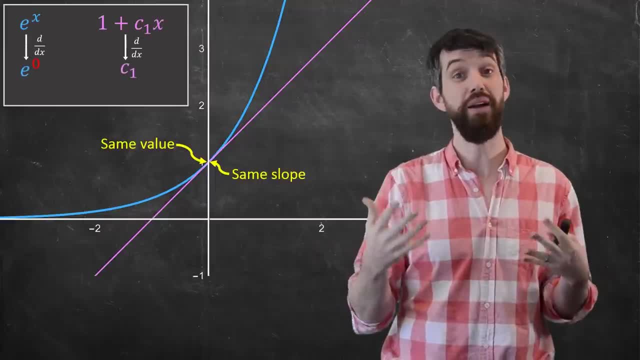 the derivative. So I'll take the derivative of both and then, if I plug 0 into that, e to the 0 is again 1, and I get that our c1 is 1 as well. So what do we have? 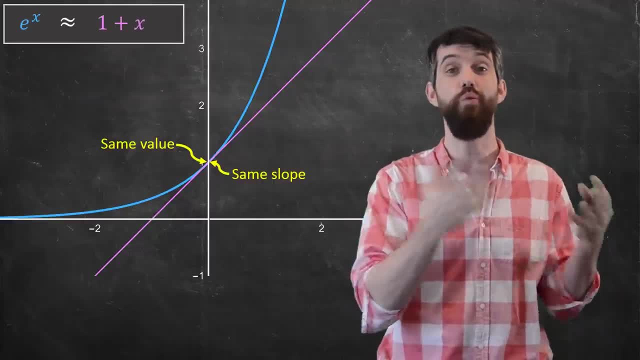 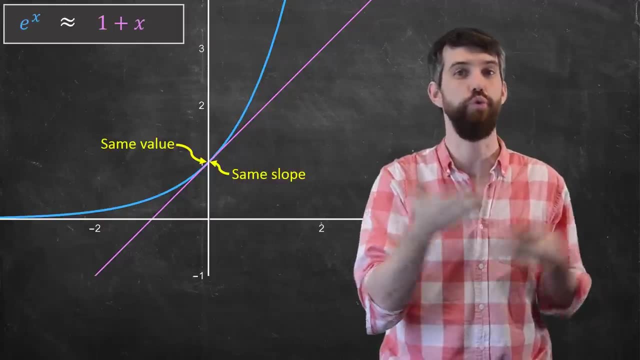 Our approximation is then that this e to the x is being approximated by 1 plus x, Which is not to say that they're exactly equal. indeed, far away from the value of 0, it becomes a worse and worse approximation, But nearby it's not bad. 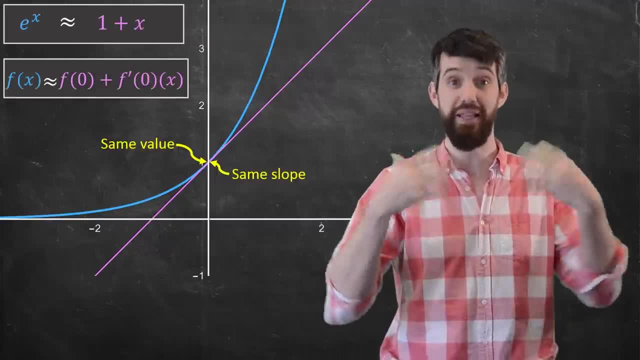 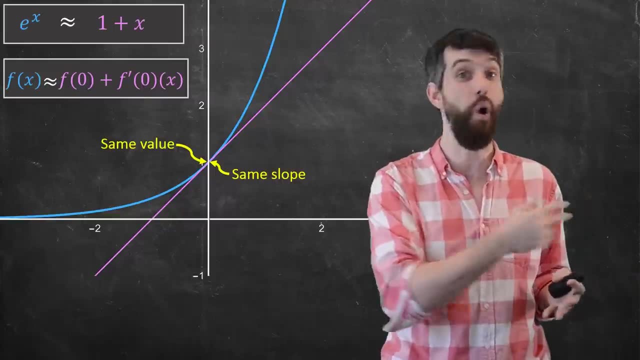 Slightly. more generally, the linear approximation is going to be that f of x is approximately f of 0 plus 0. The derivative at 0 all times x, And I'll let you recall how we did that in Calculus 1, it's the same idea of what we. 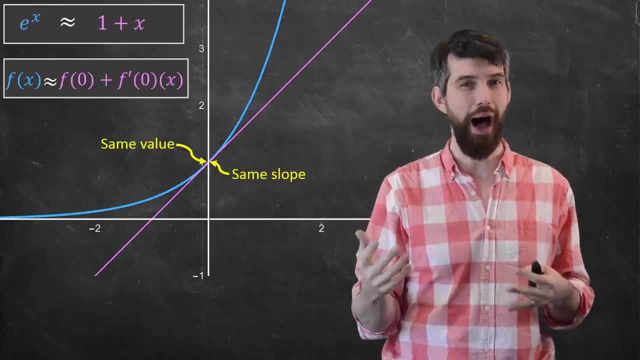 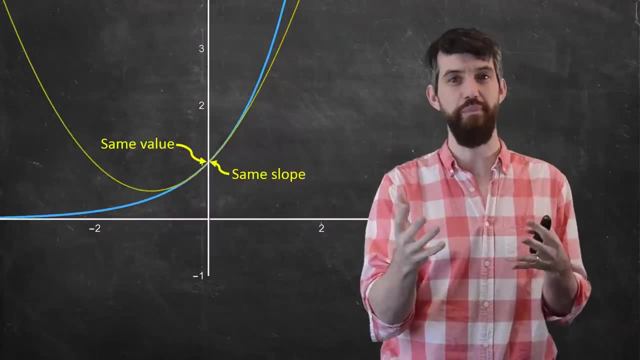 just walked through. Well, now let's go up to degree 2 polynomials. So instead of just this tangent line, I'm going to go and try to approximate it by a quadratic, And the restrictions are going to be the same: two initial ones. it has the same y value. 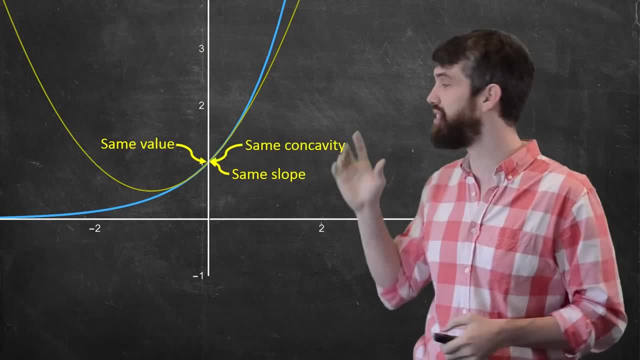 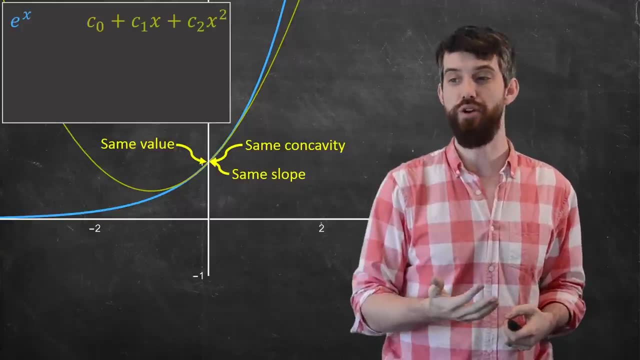 and it has the same slope. But in addition I'm going to demand that it has the same concavity, that when I've got this quadratic I've got three different restrictions on it. Then a generic quadratic can be written as a c0 plus a c1x plus a c2x squared. 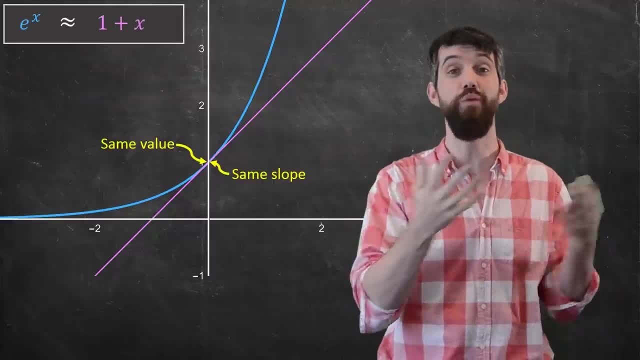 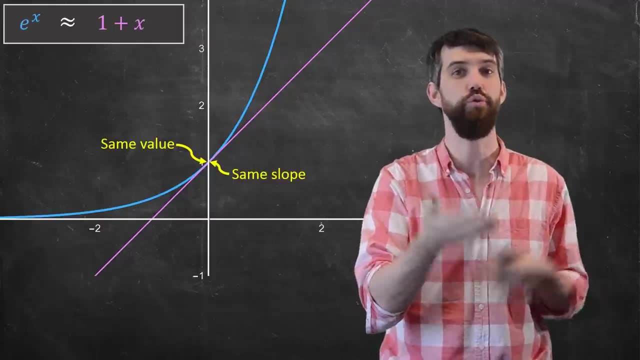 Our approximation is, then, that this e to the x has been approximated by 1 plus x, which is not to say that they're exactly equal. Indeed, far away from the value of 0, it becomes a worse and worse approximation, But nearby it's not bad. 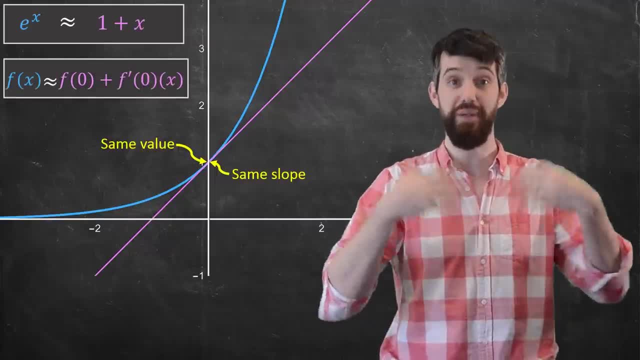 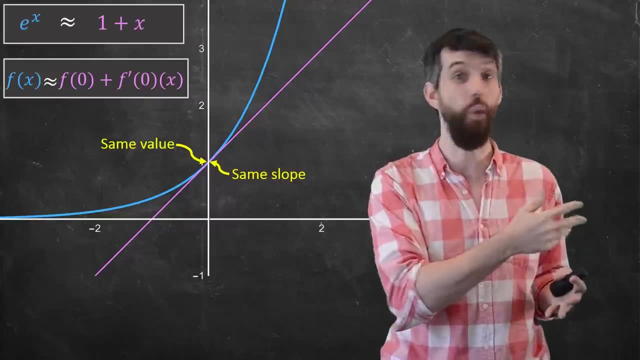 Slightly. more generally, the linear approximation is going to be that f of x is approximately f of 0 plus 1. Plus the derivative at 0, all times x. And I'll let you recall how we did that in Calculus 1.. 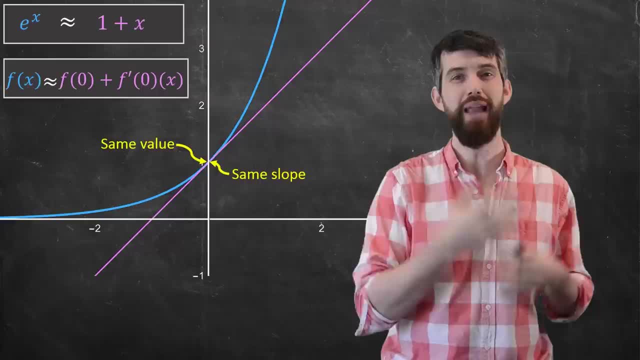 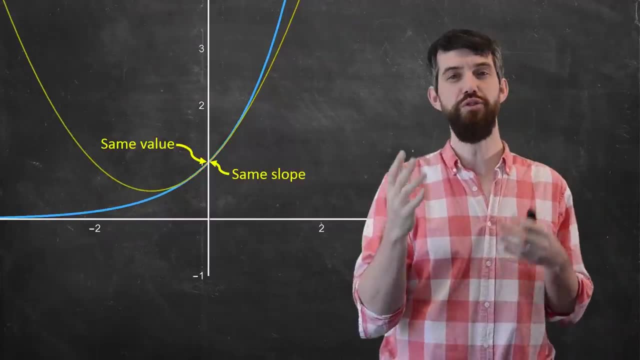 It's the same idea of what we just walked through. Well, now let's go up to degree 2, polynomials. So, instead of just this tangent line, I'm going to go and try to approximate it by a quadratic, And the restrictions are going to be the same: two initial ones. 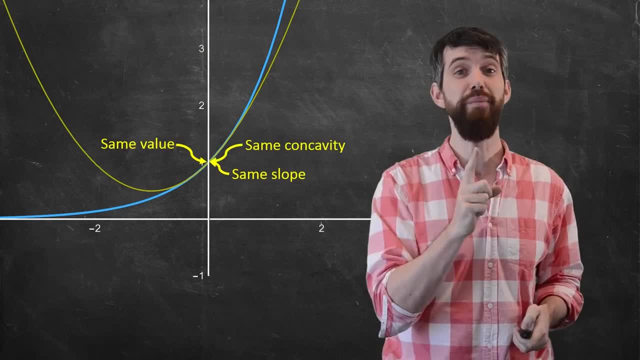 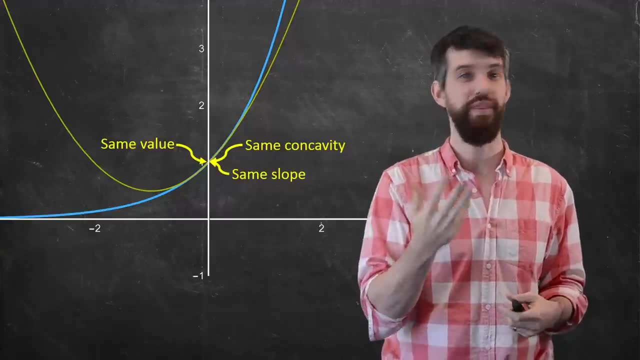 It has the same y value and it has the same slope. But in addition I'm going to demand that it has the same concavity, that when I've got this quadratic It's got three different restrictions on it. Then a generic quadratic can be written as a c0 plus a c1x plus a c2x squared. 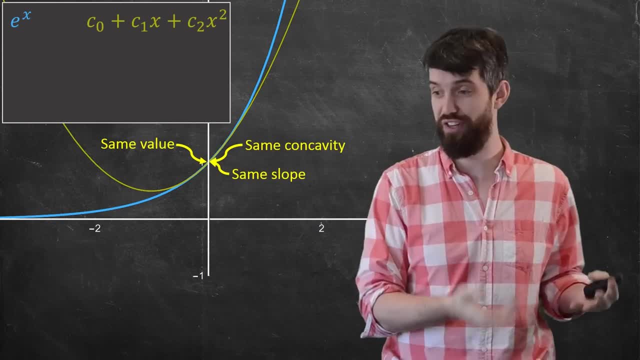 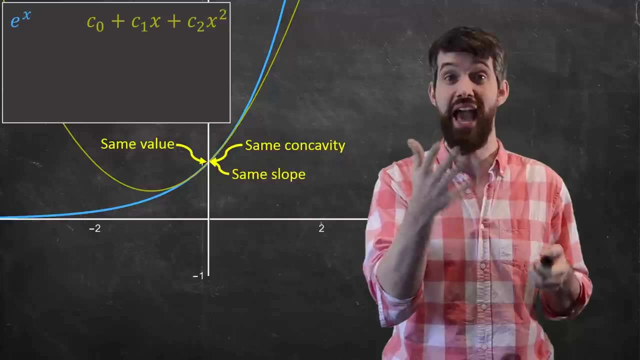 Which is to say a generic polynomial with three different coefficients. I've got three different conditions. I think it's going to work out. So same story that we did before. Let's first plug in the x equal to 0. If I do this, most of the polynomial goes away. 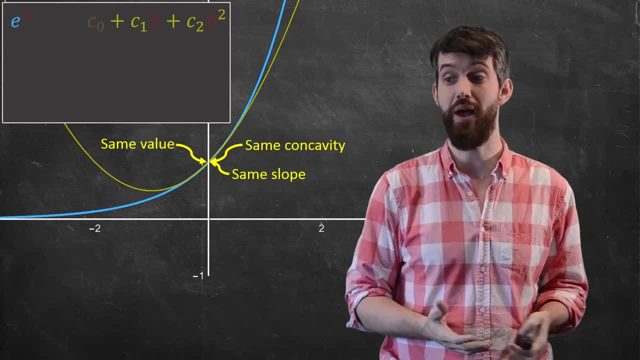 And you get e to the 0,, which is 1, is just your c0.. So I can replace my c0 with that 1.. So I can replace my c0 with that 1.. So I can replace my c0 with that 1.. 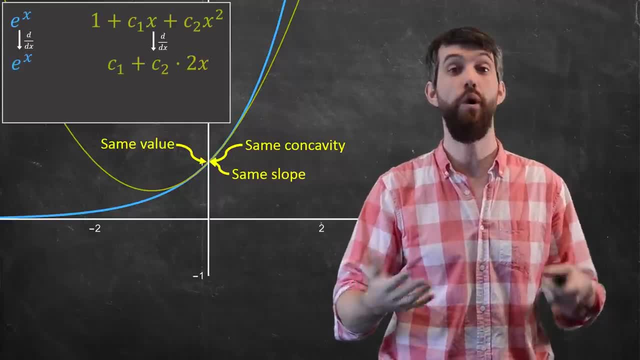 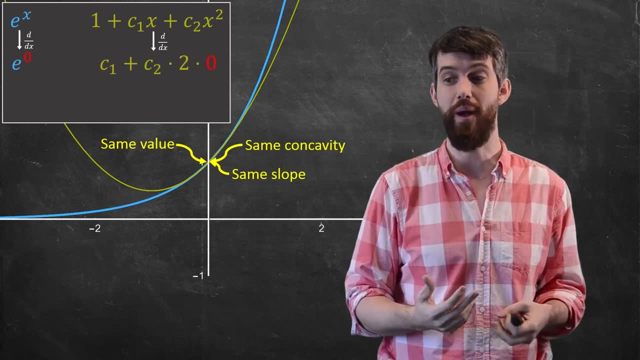 Now I'm going to take the derivative because I want the slopes to be equal on these two things. Again, I will say that this is at 0. So it's my slope being equal at x, equal to 0. So I'm going to plug in 0, and I get e to the 0,, which is 1, is c1, plus a bunch of stuff. 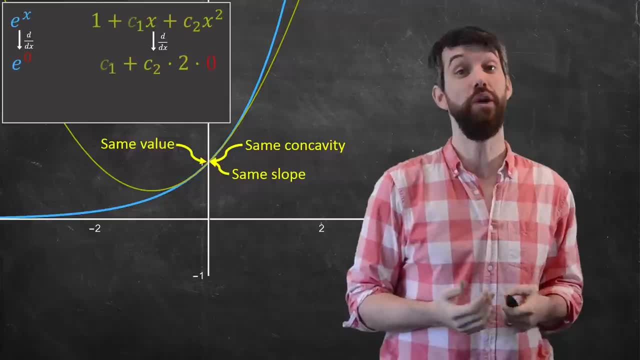 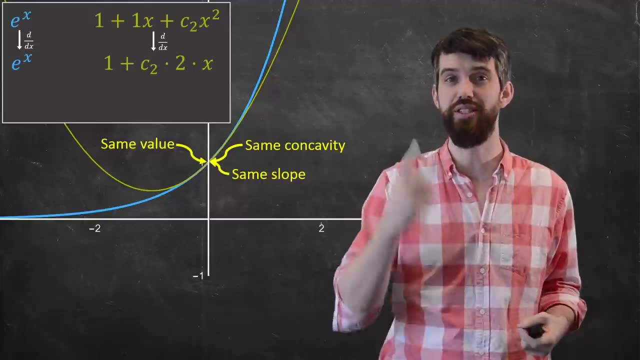 which is 0. So that tells me my c1 now is also going to be equal to the value of 1.. So I'll replace everywhere there's a c1 with a 1.. Now I want to look at concavity, which is the second derivative. 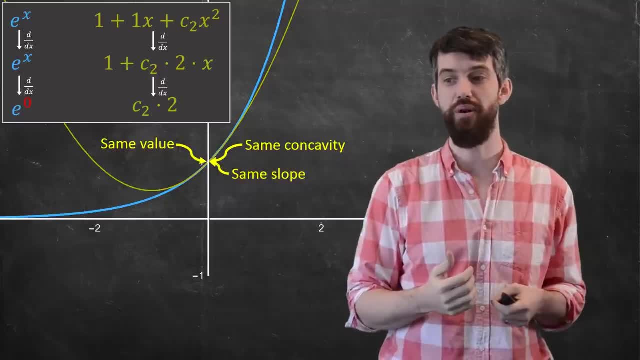 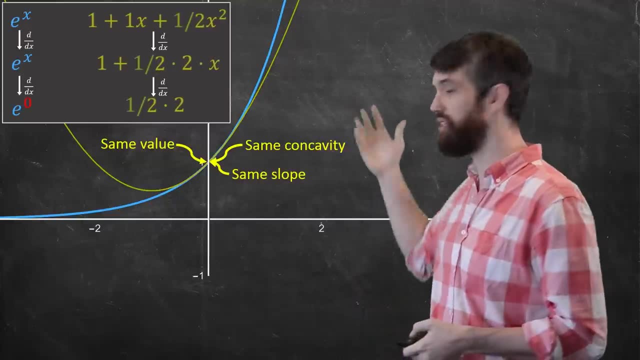 So I take the derivative one more time, I plug in x equal to 0. And what do I get? e to the 0 is 1, yet again. So c2 is 1 half and I can replace all the c2s with 1 halves, which is to say that what? 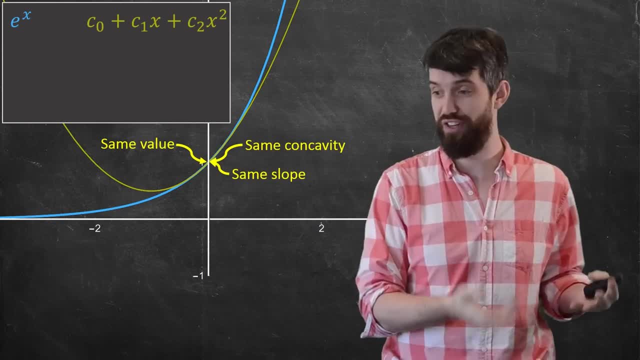 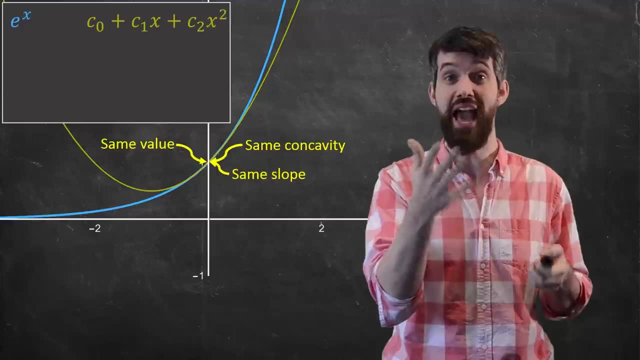 Which is to say a generic polynomial with three different coefficients. I've got three different conditions. I think it's going to work out. So same story that we did before. let's first plug in the x equal to 0. If I do this, most of the polynomial goes away. 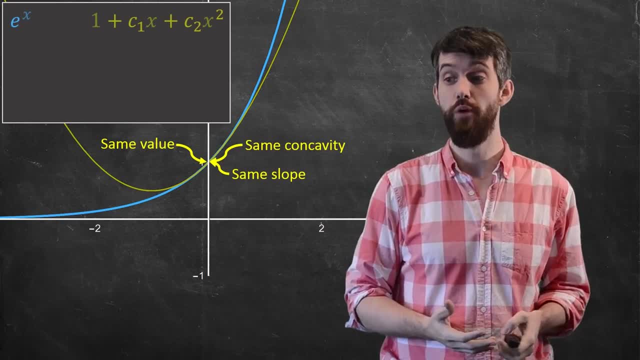 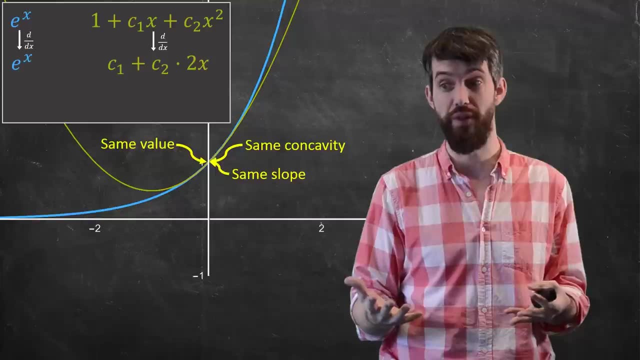 You get e to the 0,, which is 1, is just your c0. So I can replace my c0 with that 1.. That's my polynomial. Now I'm going to take the derivative because I want the slopes to be equal on these two. 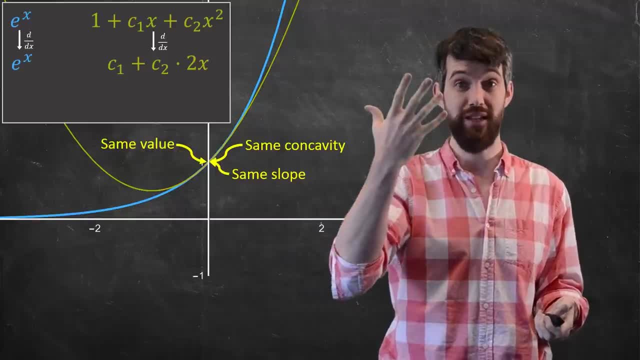 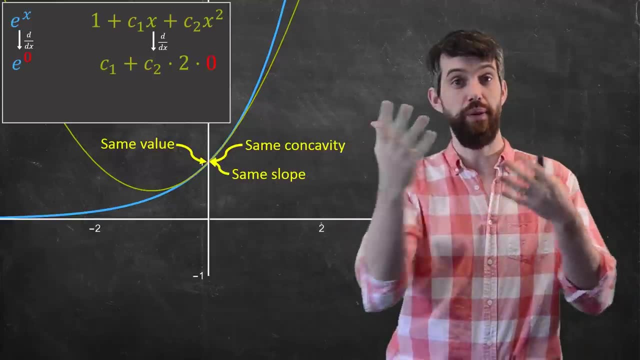 things Again. I will say that this is at 0, so it's my slope being equal at x, equal to 0. So I'm going to plug in 0 and I get e to the 0, which is 1, is c1 plus a bunch of stuff. 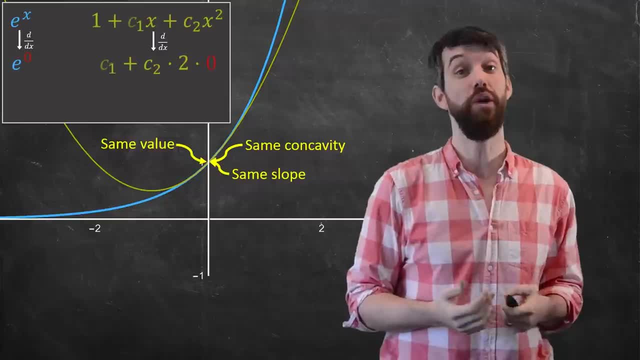 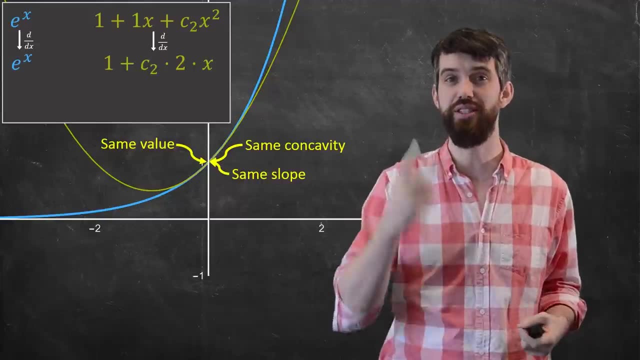 which is 0.. So that tells me my c1 now is also going to be equal to the value of 1, so I'll replace everywhere there's a c1 with a 1.. Now I want to look at concavity, which is the second derivative. 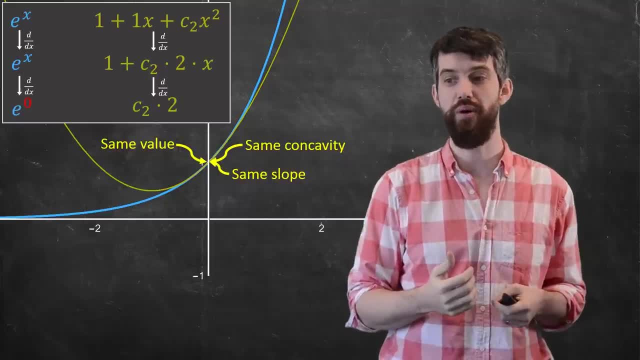 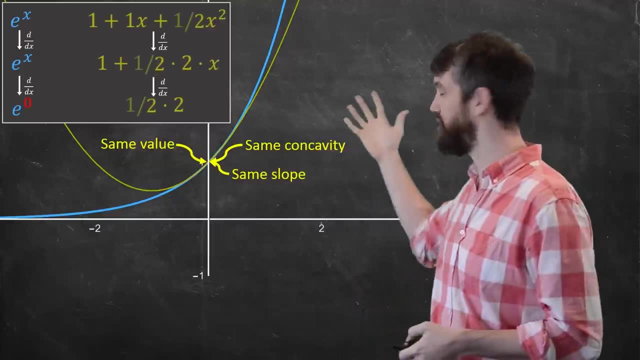 So I take the derivative one more time, I plug in x equal to 0, and what do I get? e to the 0 is 1, yet again. So c2 is 1 half and I can replace all the c2s with 1 halves, which is to say that what? 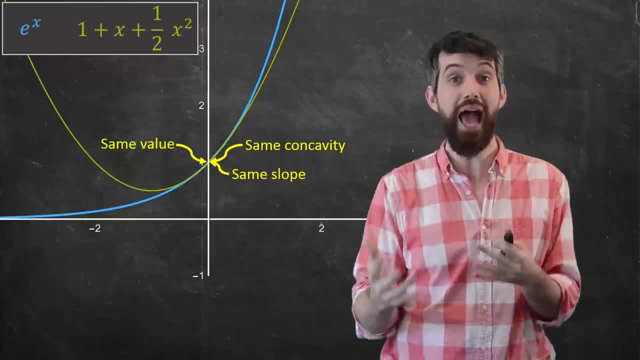 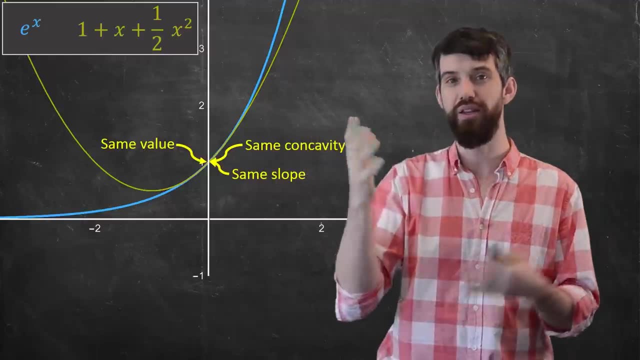 I have is this polynomial here this: 1 plus x plus 1 half x squared. That is how I came up with the quadratic that is going to well approximate near the value of x equal to 0.. Okay, this is how I did it, for e to the x. 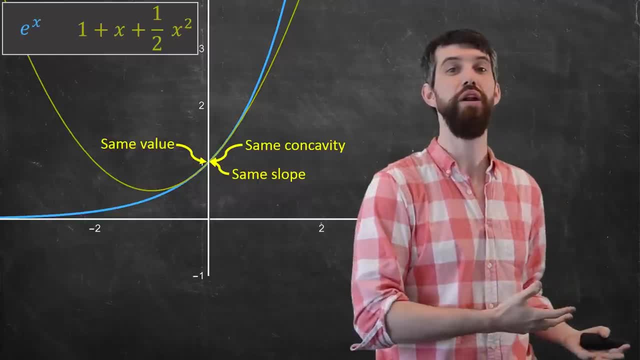 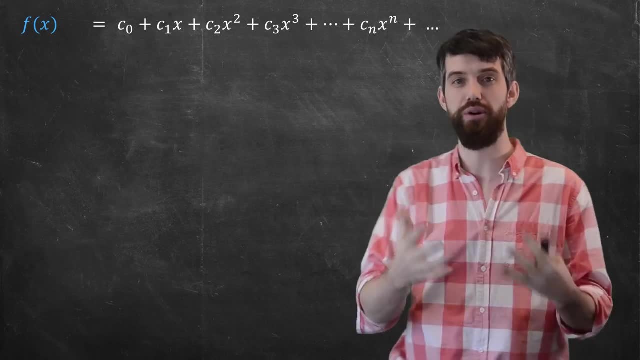 But let's take that idea And let's generalize it, Let's do it for all functions, at least functions that have power series. That is, I take a generic f of x and I set it equal to a power series and say that this 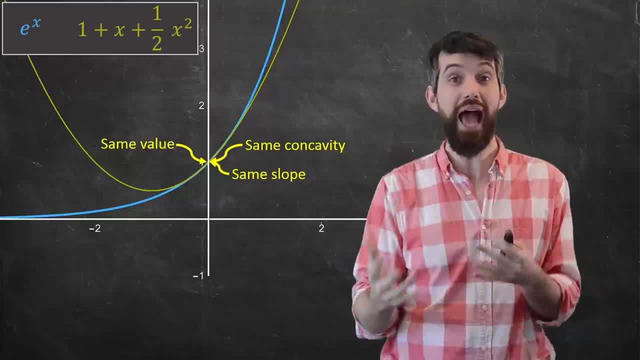 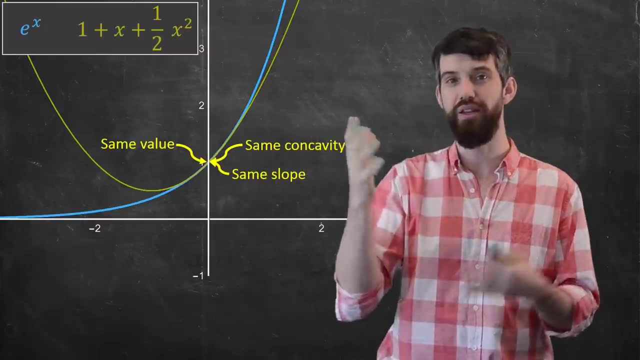 I have is this polynomial here this: 1 plus x plus 1 half x squared. That is how I came up with the quadratic that is going to well approximate near the value of x equal to 0.. OK, This is how I did it, for e to the x. 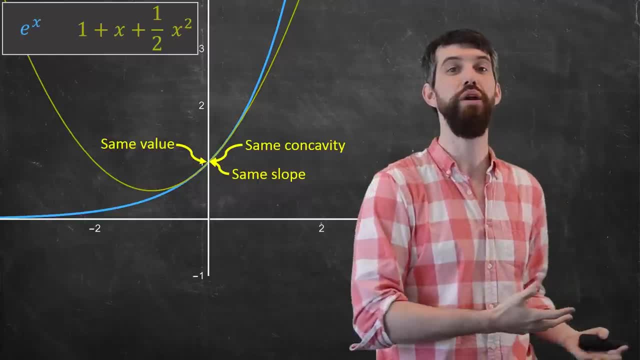 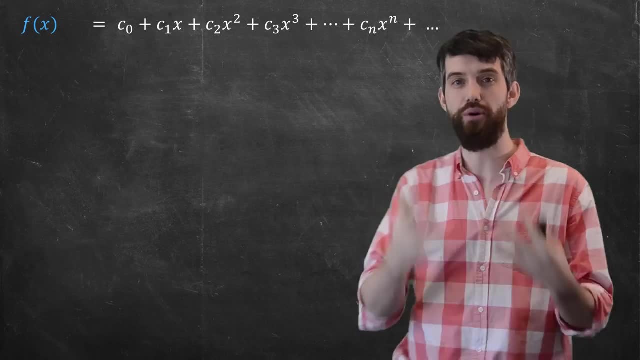 But let's take that idea And let's generalize, Let's do it for all functions, at least functions that have power series. That is, I take a generic f of x and I set it equal to a power series and say that this 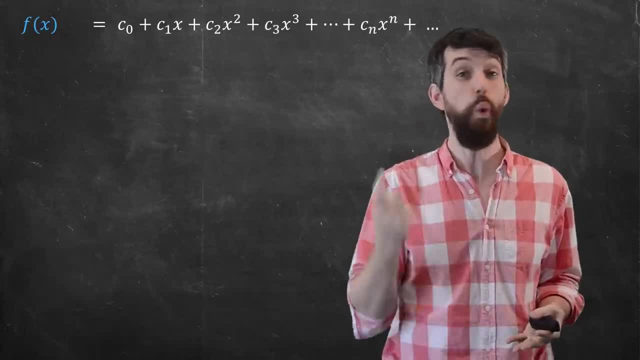 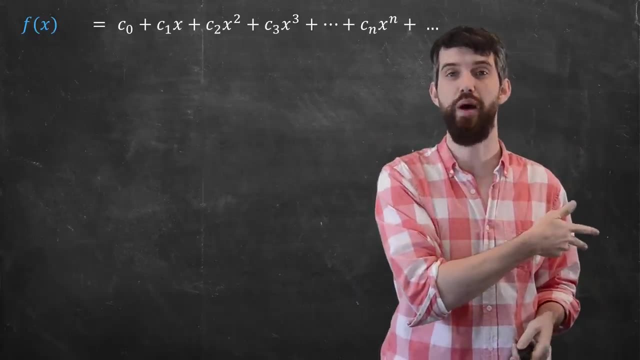 converges for some radius. And the question is: well, what are the coefficients, What are the c0, the c1, and so on? Well, let's take a few derivatives, as I did in my example with my quadratic. 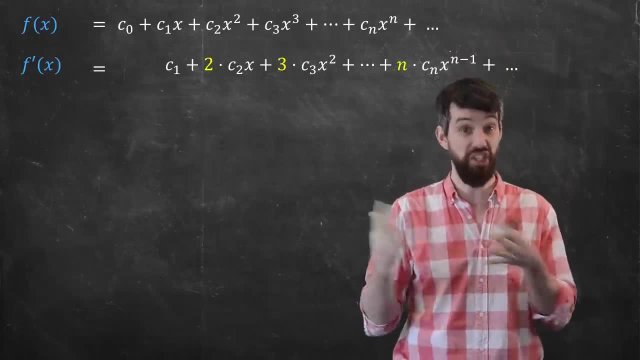 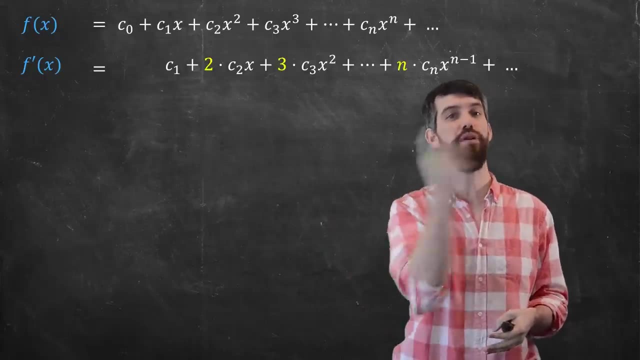 In that case, first derivative is going to mean that my c0 term goes away, My c1 x term becomes just c1. And then x squared is going to be 0. And then x squared is going to be 0. And then x squared to 2 comes down, x cubed to 3 comes down, and so on. 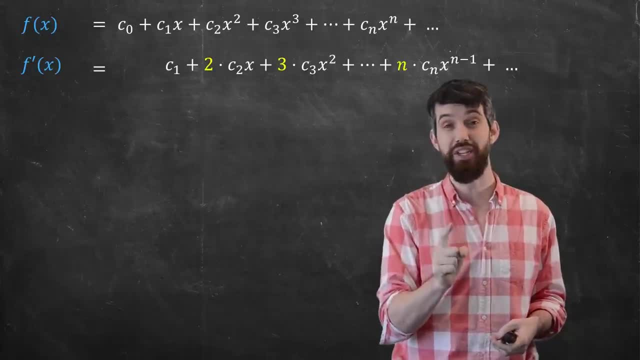 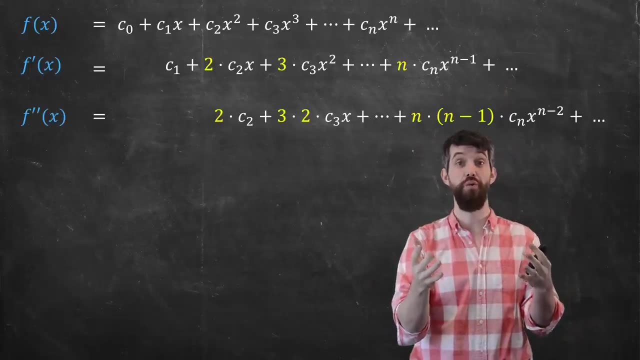 In general, the nth term, the cn x to the n. the n comes down And I'm left with this n cn x to the n minus 1.. Let's do one more derivative. So now I'm going to knock out the c1.. 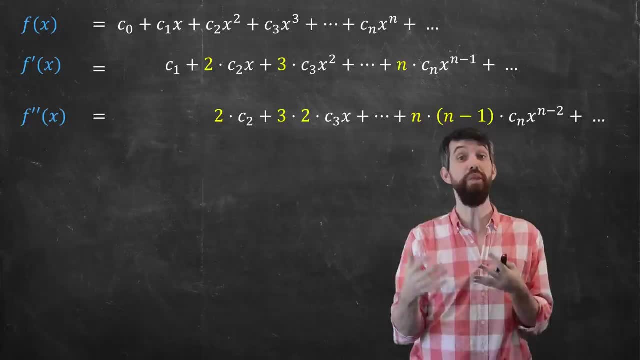 The 2- c2 is all that remains. And then, in the term that started, as x cubed, first the 3 went down and now the 2 goes down And I'm left with multiplied by x. But go to that nth term. 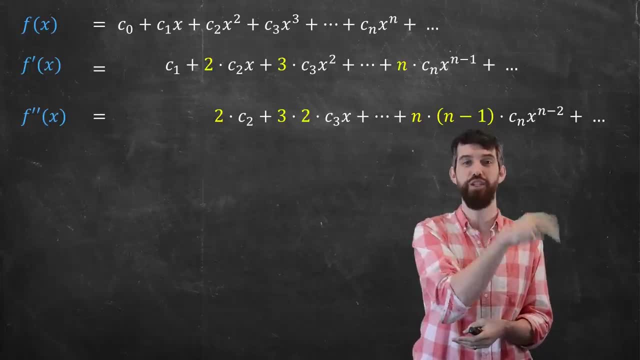 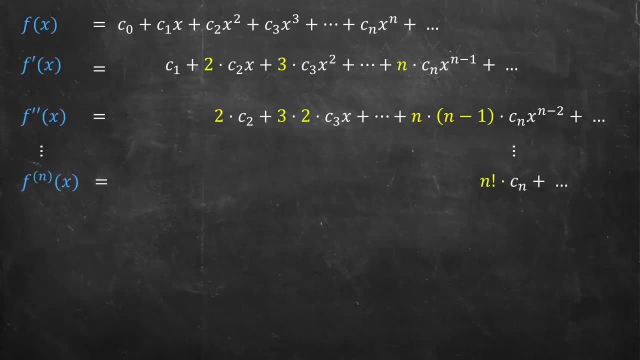 First the n came down, The first derivative. Now in the second, an n minus 1 comes down. I'm going to step away for a moment because there's not enough room, But if I take the nth derivative now, well, all the lower order terms, the terms where. 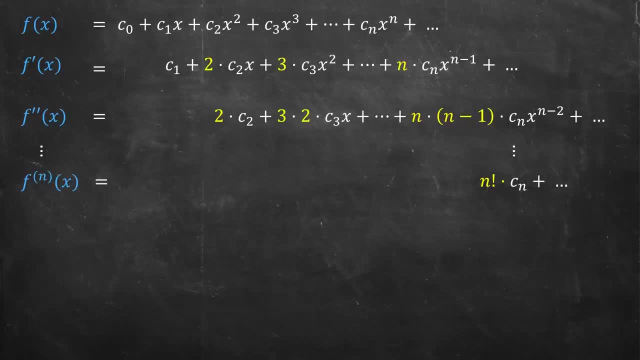 the power of x was less than n. all of those have had enough derivatives that they go to 0.. For the nth term itself, the x to the n. well, first I hang down the n, then the n minus 1, then the n minus 2.. 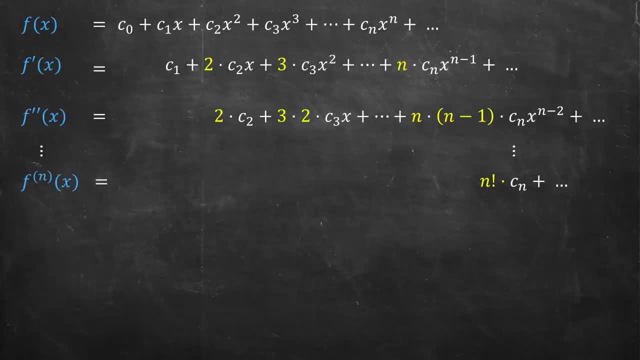 In general this is an n factorial. when I do it n times, That's just multiplied by the cn. And then I take the nth derivative, Again the x goes away, And then I have a whole bunch of more higher order terms where the x's remain. 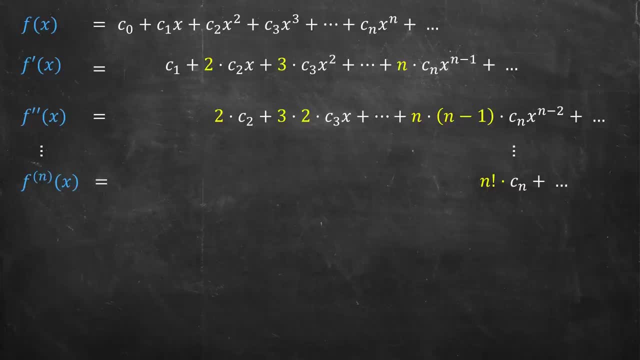 Now, after taking derivatives. well, what did we do previously? We plugged it in x equal to 0. So let's, everywhere there's an x, I'm going to replace this with a 0.. Now this gives me a series of equations. 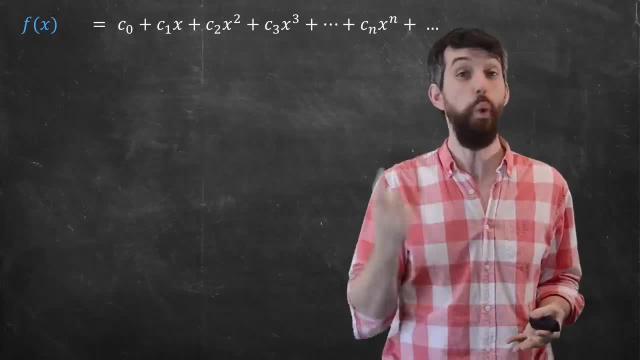 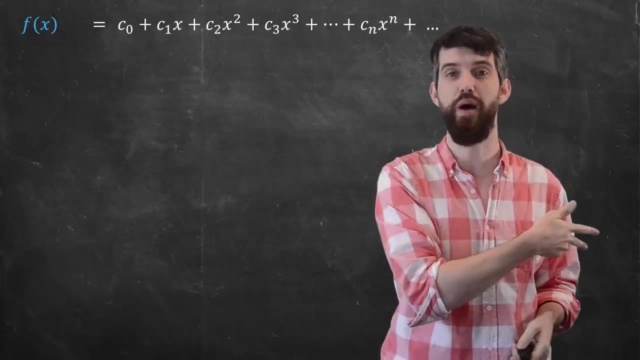 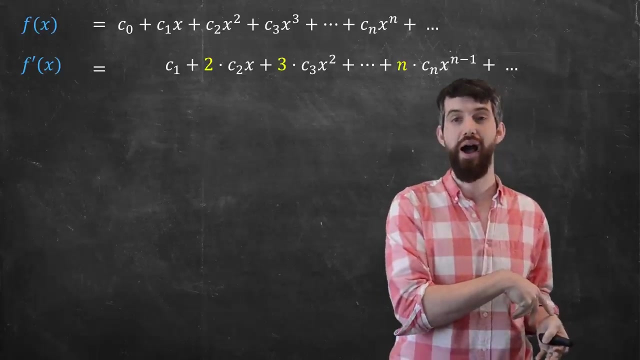 converges for some radius. And the question is: well, what are the coefficients, What are the c0, the c1, and so on? Well, let's take a few derivatives, as I did in my example with my quadratic. In that case, first derivative is going to mean that my c0 term goes away, my c1 x term. 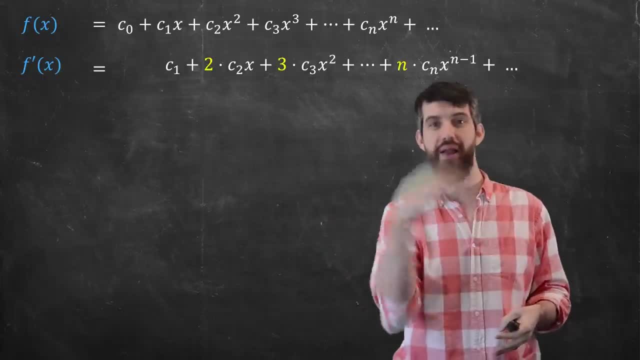 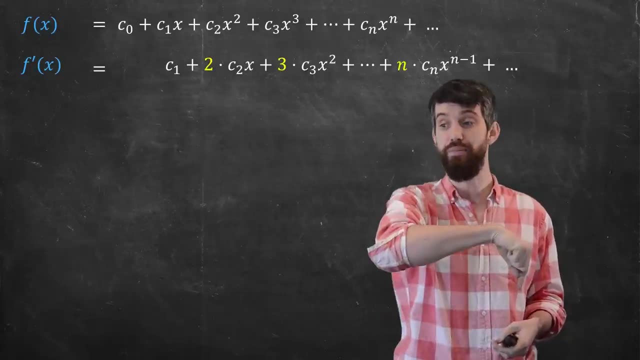 becomes just c1.. And then x squared to 2 comes down, x cubed to 3 comes down, and so on. In general, the nth term, the cn, x to the n, the n comes down and I'm left with this n. 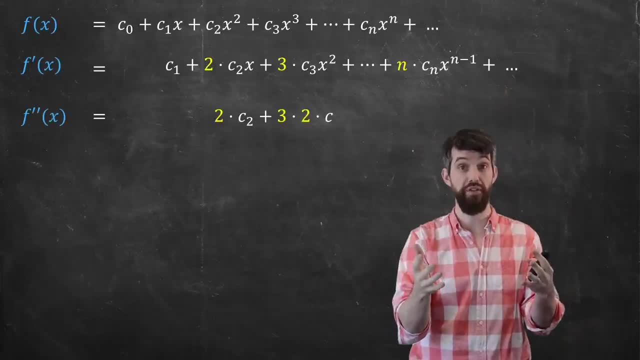 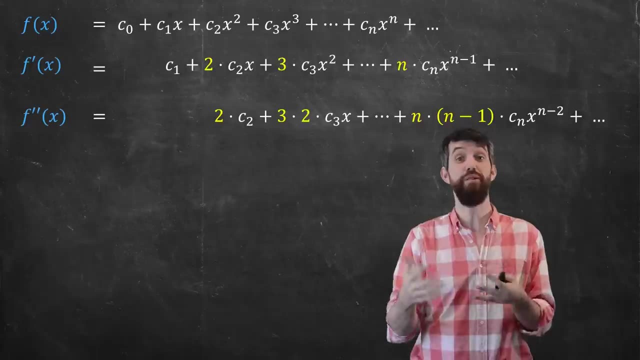 cn, x to the n minus 1.. Let's do one more derivative. So now I'm going to knock out the c1, the 2, c2 is all that remains. and then, in the term that started, as x cubed, first the 3 went down and now the 2 goes down and I'm left. 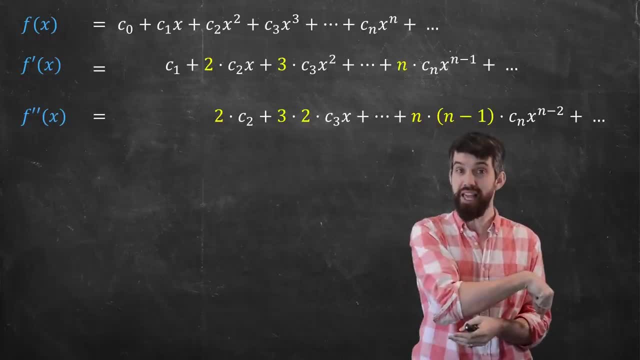 with multiplied by x, But go to that nth term. First the n came down, the first derivative, and now in the second an n minus 1 comes down. I'm going to step away for a moment because there's not enough room, but if I take the, 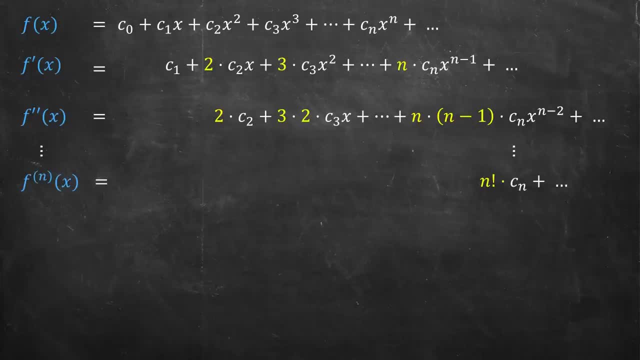 nth derivative now. well, all the lower order terms, the terms where the power of x was less than n, all of those have had enough derivatives that they go to 0.. For the nth term itself, the x to the n. well, first I hang down the n, then the n minus. 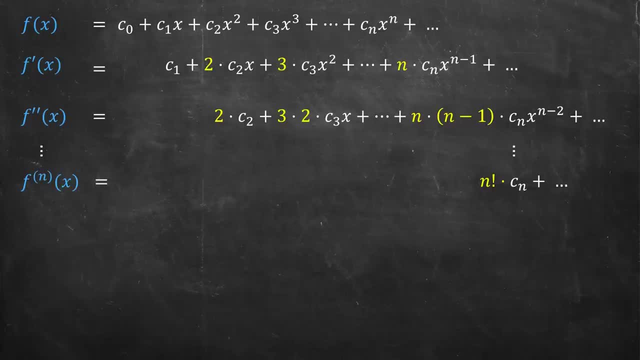 1, then the n minus 2.. In general this is an n factorial one I do at n times. That's the n, That's just multiplied by the cn, the x goes away, And then I have a whole bunch of more higher order terms where the x's remain. 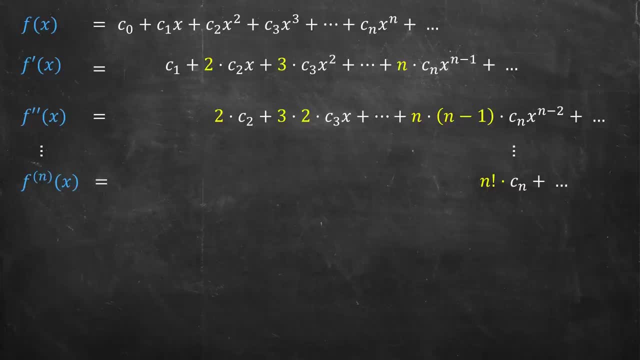 Now, after taking derivatives. well, what did we do previously? We plugged it in x equal to 0. So let's, everywhere there's an x, I'm going to replace this with a 0.. Now this gives me a series of equations. I can compute what all the different c values. 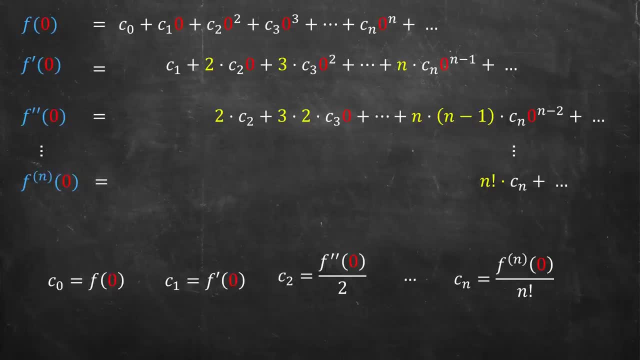 are. So for the first line, every single thing except for c0 is indeed 0,. so c0 is just f of 0. Everything about the first remaining coefficient, c1, is 0. So c1 is just f prime of 0. 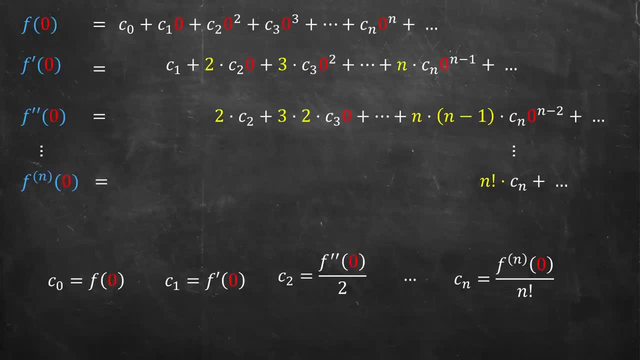 c2 is f, double prime at 0 over 2.. And generically, cn is you take n derivatives of it and then you divide out by this n factorial thing to make it balance. By the way, these first few terms I can interpret in the language of factorials: 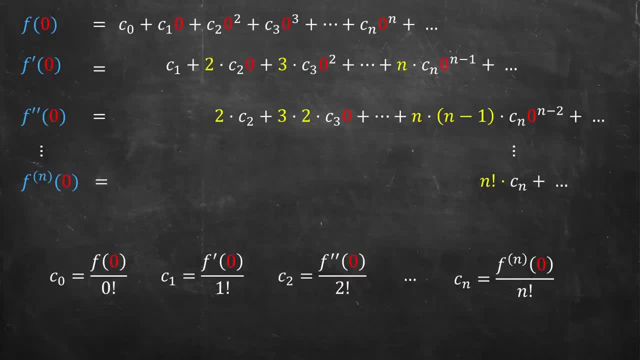 0- factorial is just 1,. 1- factorial is just 1,, 2- factorial is just 2, so I can replace those coefficients in the denominator, And so it's quite compatible with the generic. In the generic form you take n derivatives and divide it by n- factorial. 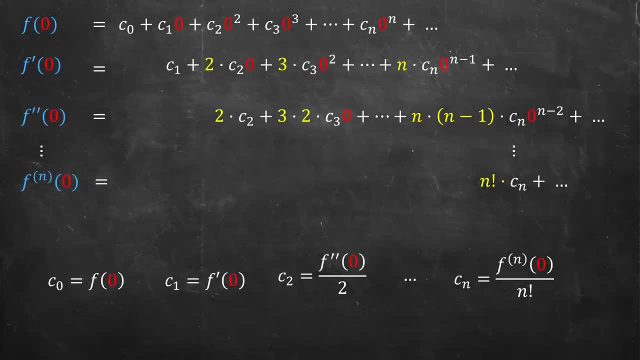 I can compute what all the different c values are. So for the first line, every single thing except for c0 is indeed 0. So c0 is just f of 0.. For the second, Everything. For the first remaining coefficient, c1 is 0. 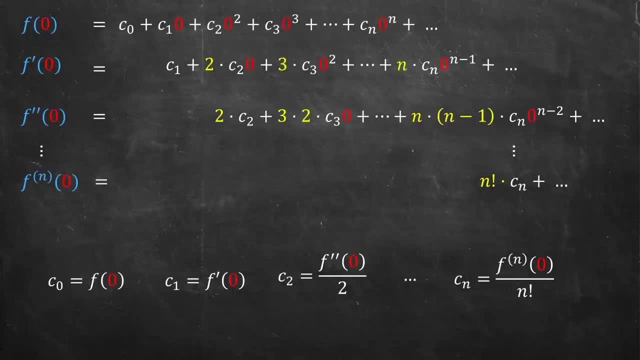 So c1 is just f prime of 0.. c2 is f double prime at 0 over 2.. And generically cn is. you take n derivatives of it and then you divide out by this n factorial thing to make it balance. 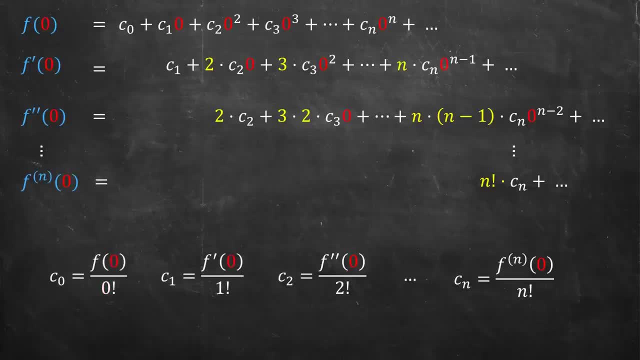 By the way, these first few terms I can interpret in the language of factorials: 0 factorial is just 1.. 1 factorial is just 1.. 2 factorial is just 2.. So I can replace those coefficients in the denominator. 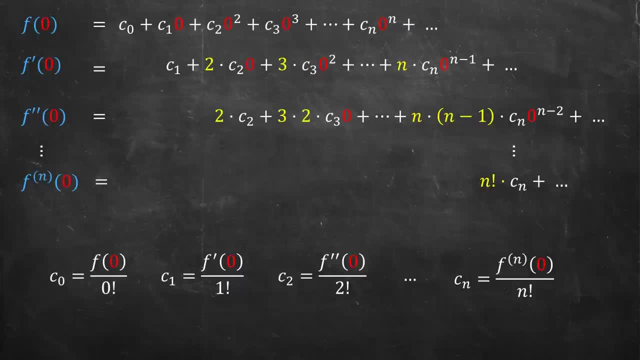 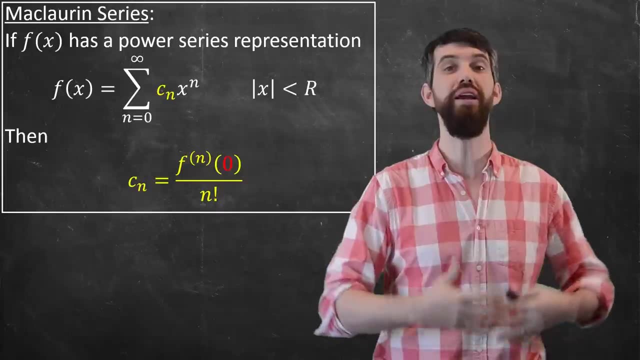 And so it's quite compatible with the generic form. You take n derivatives and divide it by n factorial. Indeed, A Maclaurin series is one where you're doing a power series around x equal to 0. You compute out what the coefficients are. 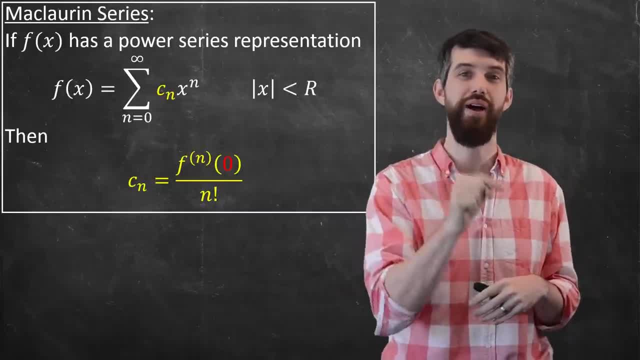 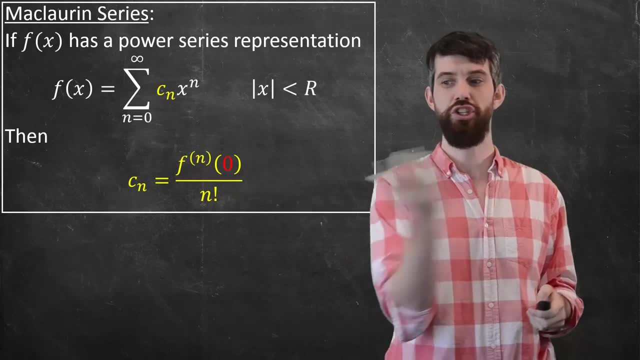 And indeed you get precisely this: These n derivatives at 0 divided by n factorial. The fact that I plugged in x equal to 0 here is in a sense unimportant. I can actually just shift this. So everywhere there's a 0, I can put it in an a. 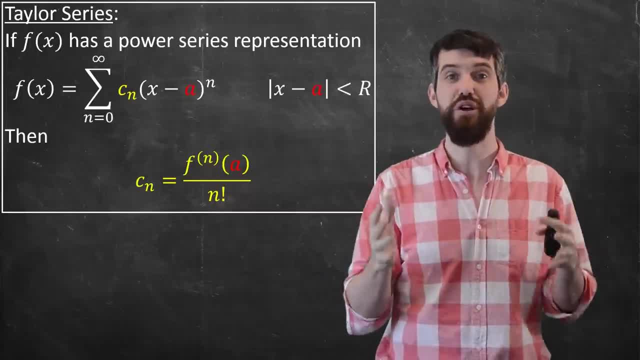 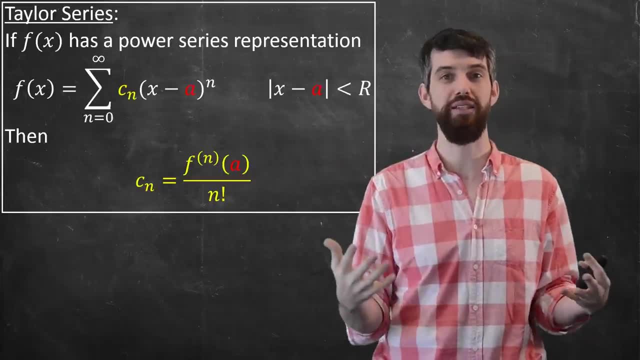 So it's x minus a And the radius is the absolute value of x, of x minus a, less than r, and the derivative is a value added a. So it's just a slight shift and in that more general case I call it a Taylor series, A Maclaurin series, where a is zero is just a. 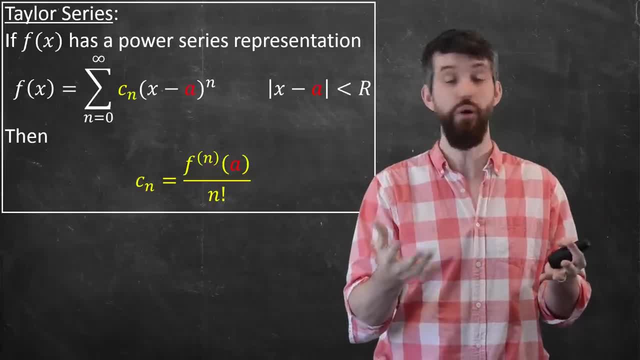 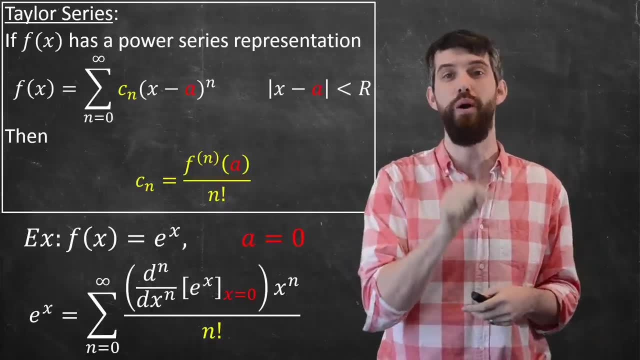 special case of the true thing: Taylor series. Okay, so let's look at that example that we had before. We started with e to the x and I'm doing it around, a equal to zero. Zero is the spot where I'm approximating it. Then, if I plug into my big gnarly formula, all right, in place of the nth. 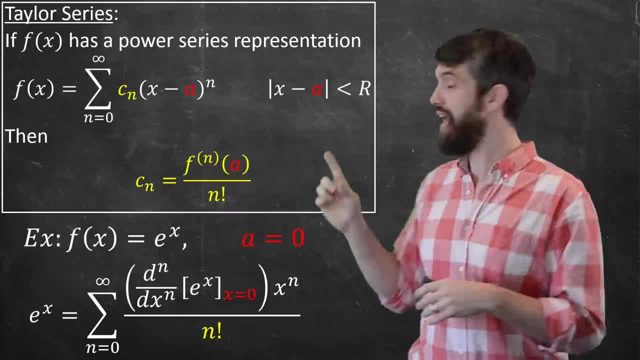 derivative. I've written it down here in Leibniz notation: the nth derivative of e to the x, evaluated at zero. But for e to the x the first derivative is e to the x. the second derivative is e to the x. 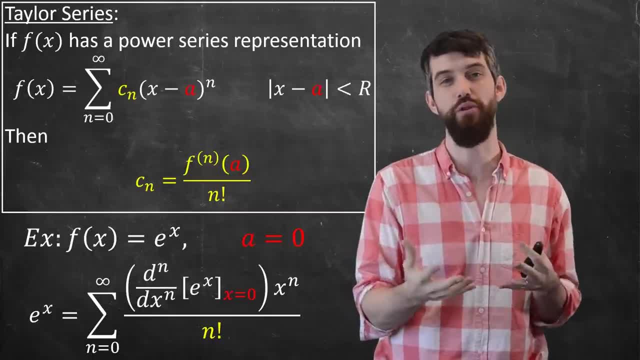 this e to the x is all the way along, so it's just e to the x. when I take n derivatives, Plugging in zero, it's e to the zero, which is one. so all of that mess goes away and I'm just left with x to. 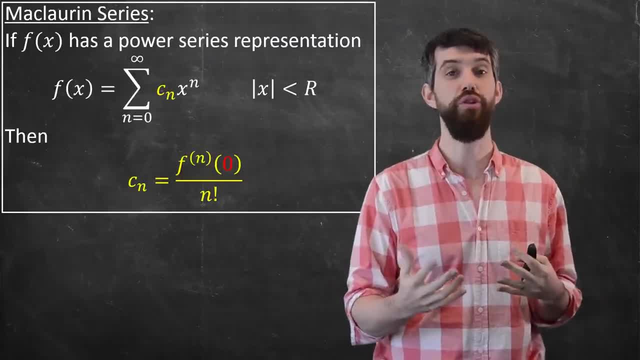 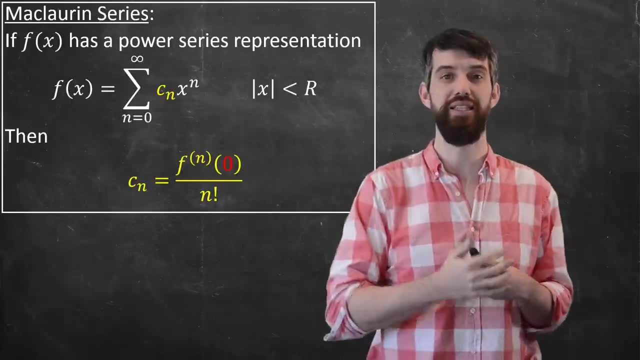 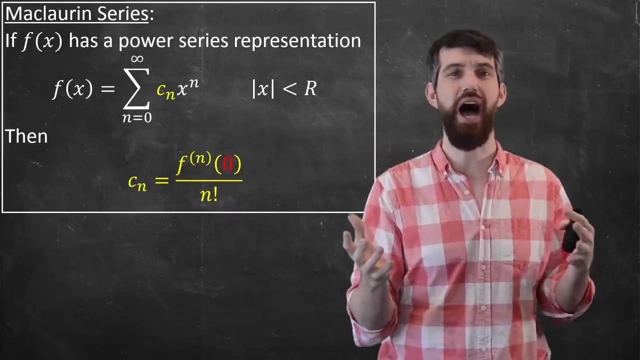 Indeed, A Maclaurin series is one where you're doing a power series around x equal to 0, you compute out what the coefficients are and indeed you get precisely this: these n derivatives at 0 divided by n factorial. The fact that I plugged in x equal to 0 here is, in a sense, unimportant. 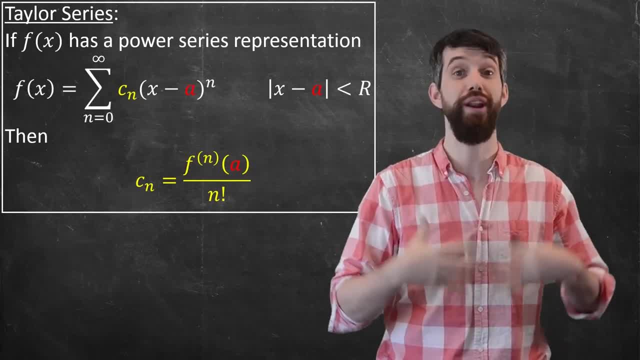 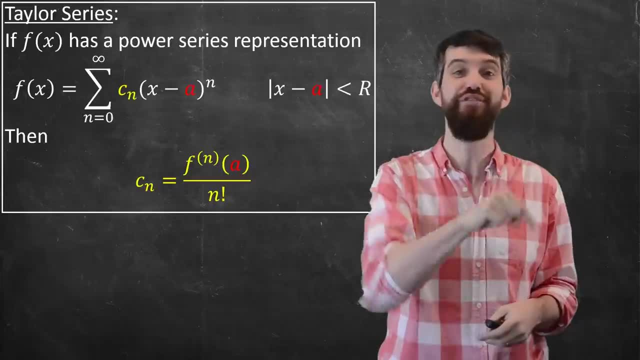 I can actually just shift this, so everywhere there's a 0 I can put in an a, so it's x minus a. This is the absolute value of x minus a less than r, and the derivative is a value at a. So it's just a slight shift and in that more general case I call it a Taylor series. 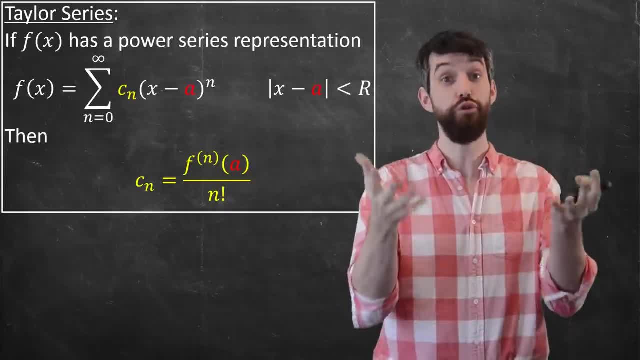 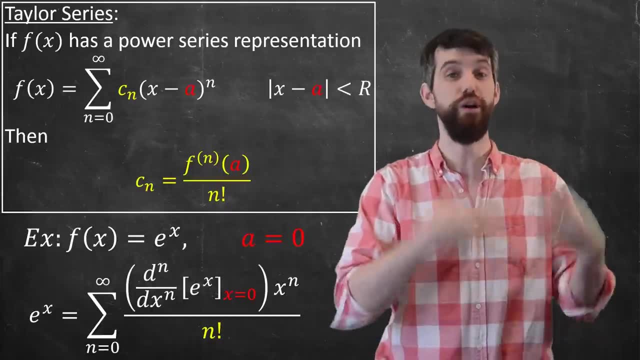 A Maclaurin series where a is 0 is just a special case of the true thing. Taylor series: Okay, so let's look at that example that we had before We started, with e to the x- and I'm doing it around- a equal to 0. 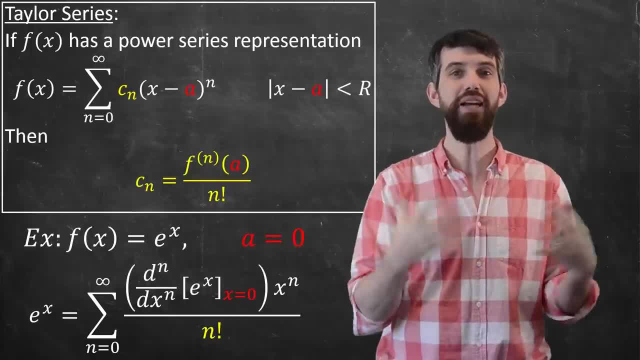 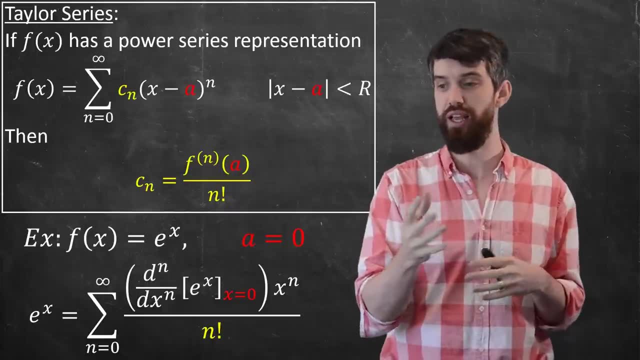 0 is the spot where I'm approximating it. Then if I plug into my big gnarly formula, Alright, In the place of the nth derivative- I've written it down here in the Liebesnotation- the nth derivative of e to the x evaluated at 0.. 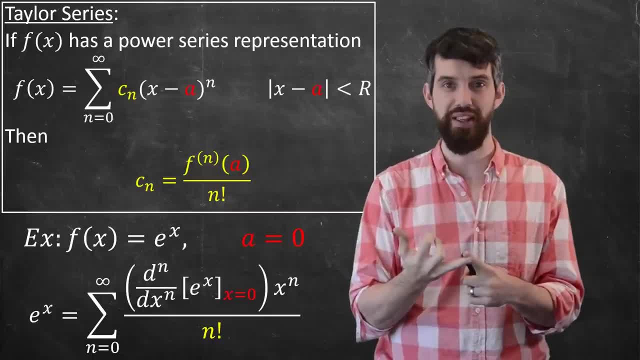 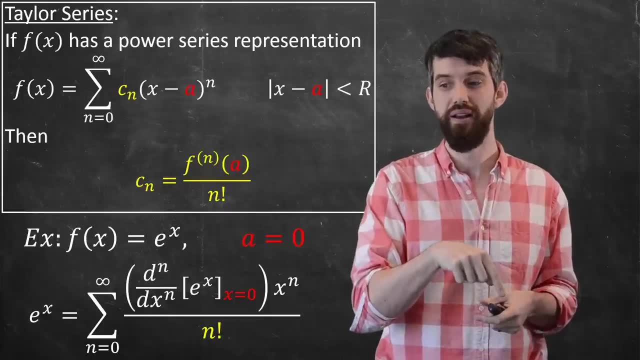 But for e to the x, the first derivative is e to the x, the second derivative is e to the x. this e to the x is all the way along, So it's just e to the x. when I take n derivatives, Plug it in to 0, it's e to the 0, which is 1.. 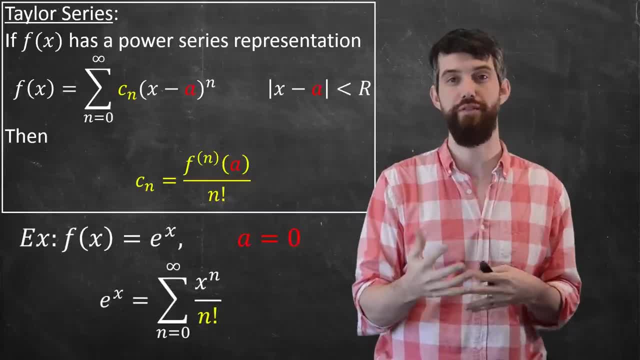 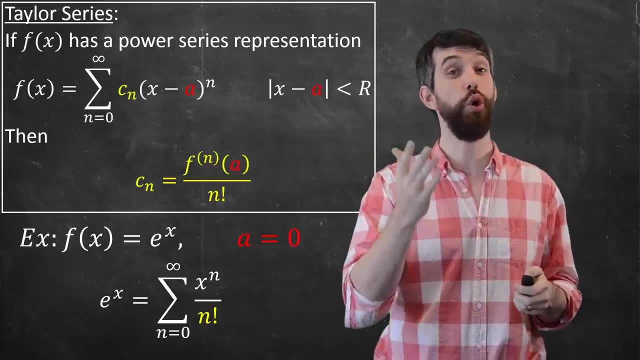 So all of that mess goes away and I'm just left with x to the n over n factorial. So this is the Taylor series for e to the x. Final thing I want to do is show up the graph now of e to the x. 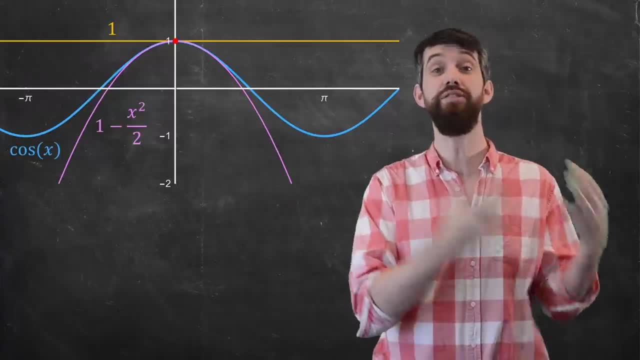 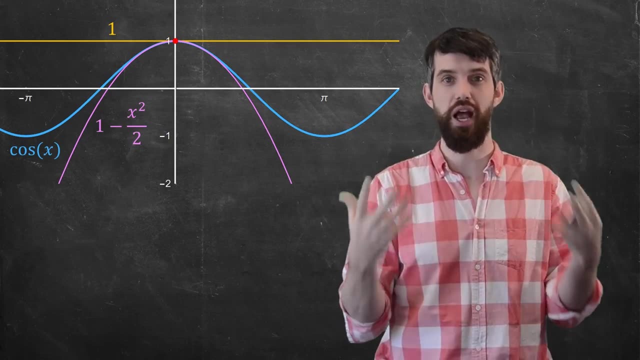 See, it's 4.. Okay, cosine with its first and second Taylor polynomial approximation. So this is the blue cosine. and then I have the tangent line to cosine, which is just the line y equal to 1, and the quadratic approximation, which is 1 minus x squared over 2.. 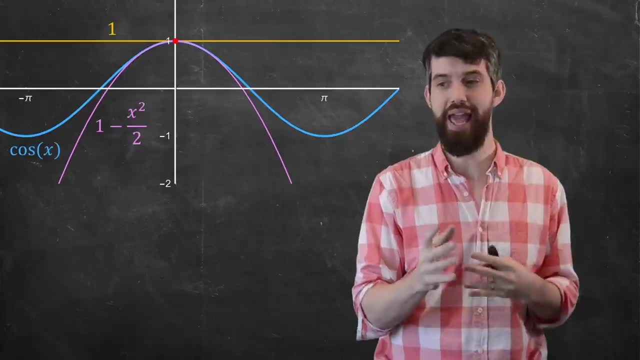 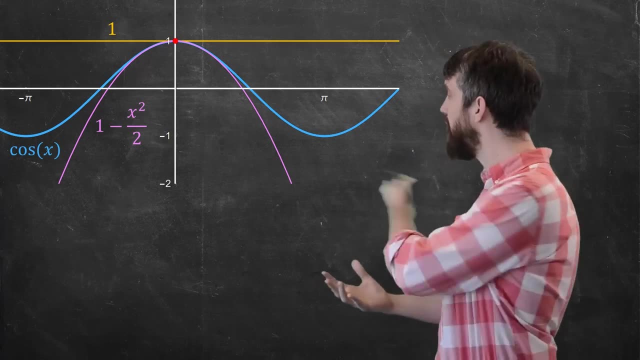 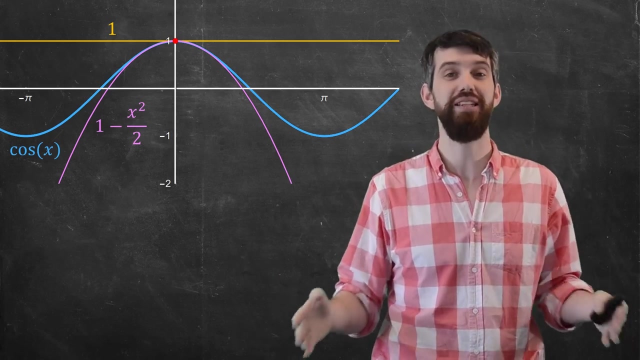 Now, what I want to notice is that this critically depends on the fact that I am doing this approximation about a equal to 0.. Indeed, these approximations look pretty good for values near 0, the quadratic one in particular, but far away, I mean quadratic is dropping off to minus infinity. far away, it's going to be a terrible approximation. 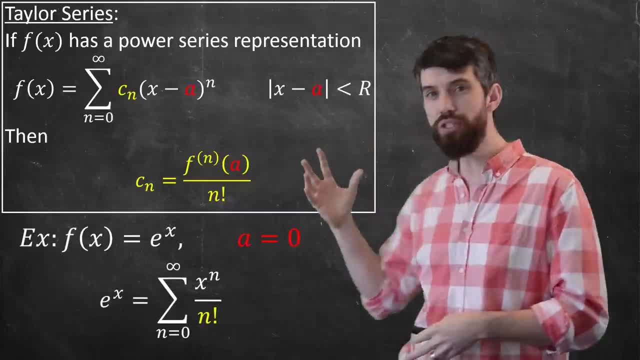 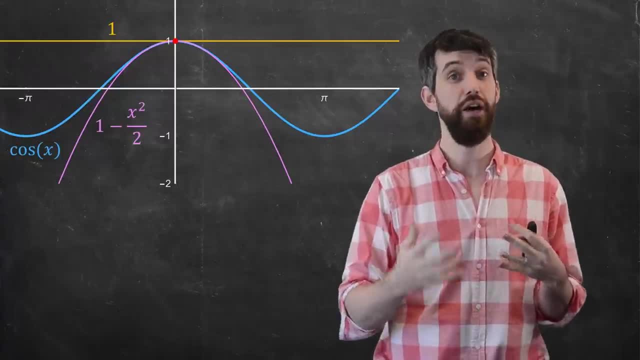 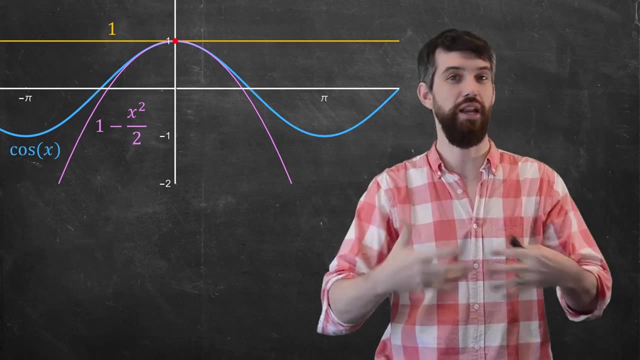 the n over n factorial. So this is the Taylor series for e to the x. Final thing I want to do is show up the graph now of cosine. So this is the blue cosine, and then I have the tangent line to cosine, which is just the line y. 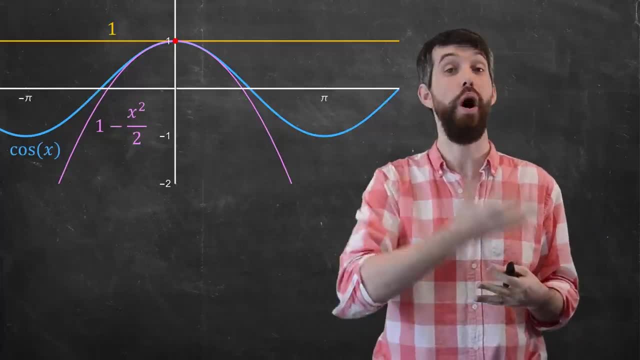 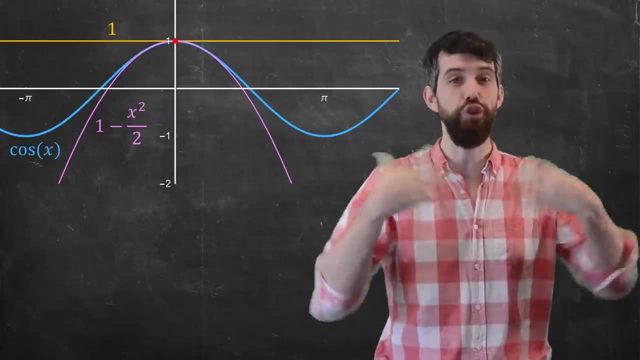 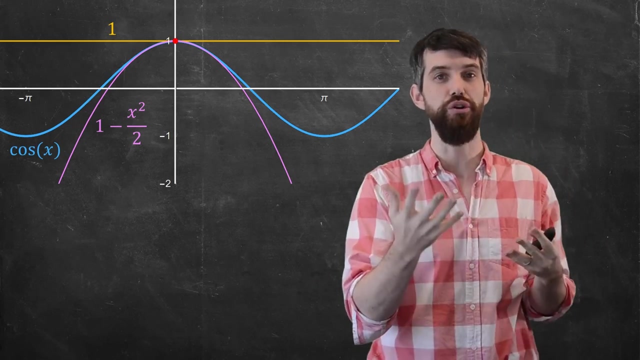 equal to 1, and the quadratic approximation, which is 1 minus x squared over 2.. Now, what I want to notice is that this critically depends on the fact that I am doing this approximation about a equal to zero. Indeed, these approximations look pretty good for values near zero. the quadratic one in: particular, but I don't want to go into too much detail on that, So I'm just going to show up the blue cosine and then I have the tangent line to cosine, which is just the line y equal to 1, and the quadratic one in particular, but I don't want to go into too much detail on that, So I'm just going. 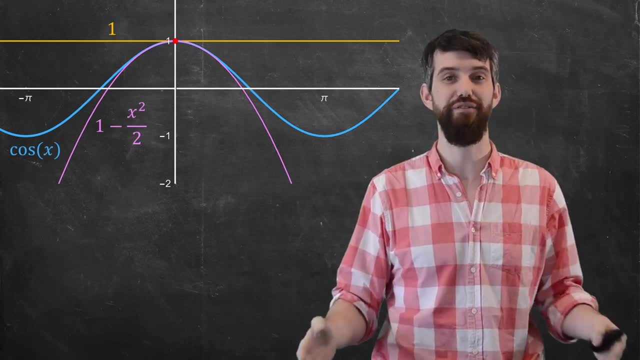 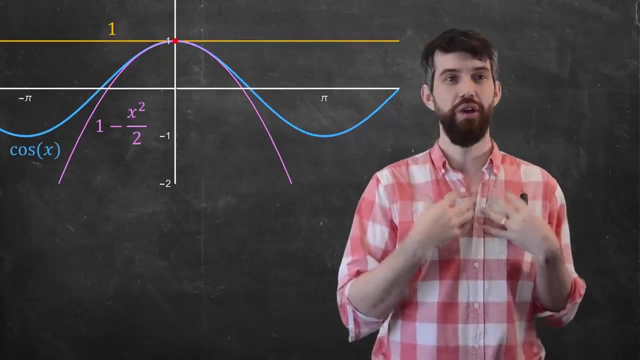 far away. I mean, quadratic is dropping off to minus infinity far away. it's going to be a terrible approximation. Now, what is fascinating about Taylor series to me is that the computation only depended the derivative exactly at the point a equal to zero. That's the only thing you needed. 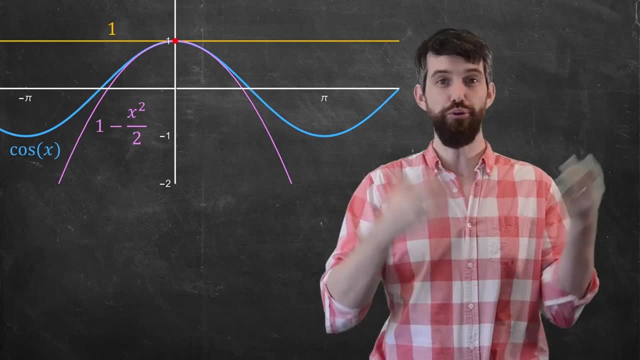 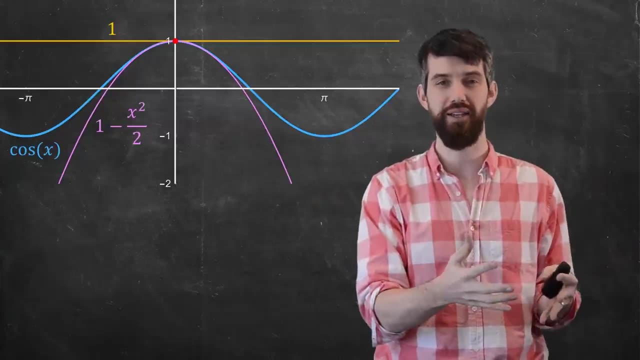 to know, But when I graph these it's a pretty good approximation, not exactly at zero, but nearby There's a sort of a whole region where it's pretty nice. We haven't quantified yet exactly what we mean by pretty nice, but it's a pretty good approximation. 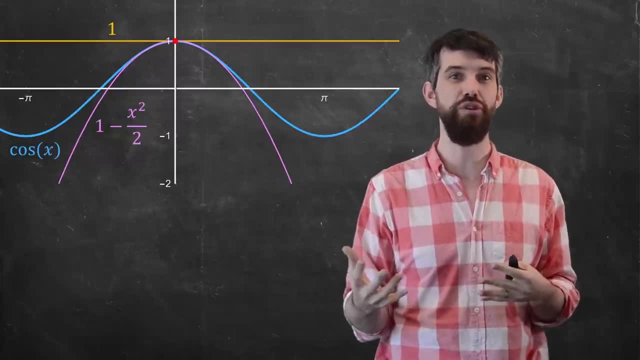 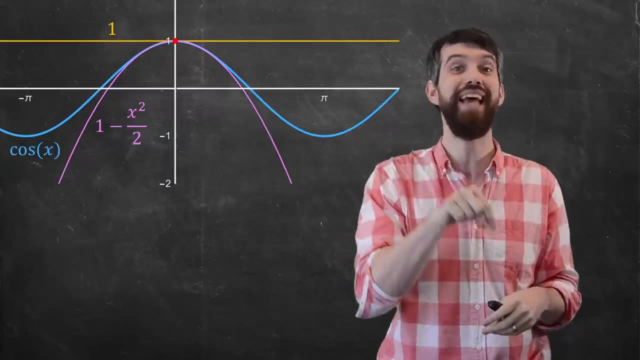 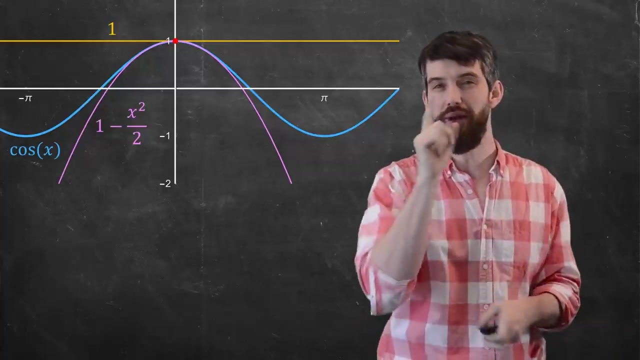 But the general idea that you're using information all taken at one point to get an approximation nearby, you get local information from this exactly one point- is an incredibly powerful and broad idea And indeed, if I now change that point, so instead of a equal to zero, 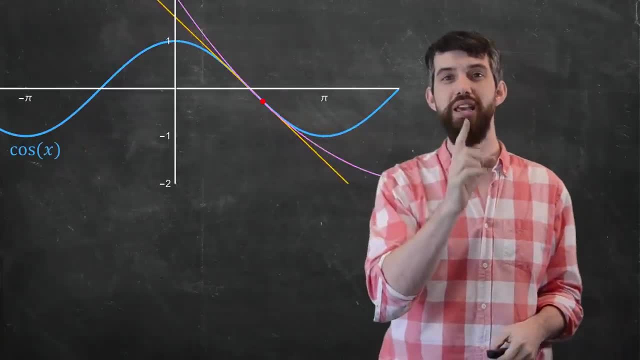 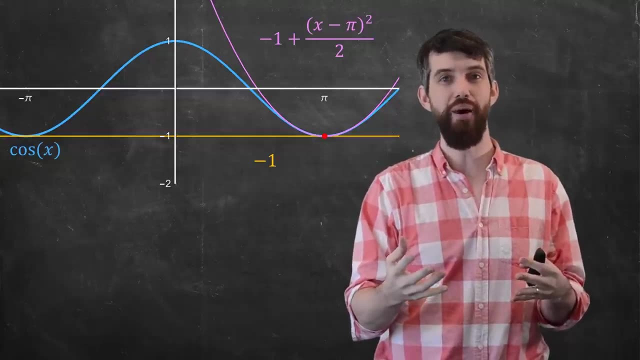 let's just move it over. Let's move it down to a equal to pi And you can see how the quadratic and the linear approximations change with it. You get now a different quadratic that approximates this at this different point and near the value of a equal to pi. it's. 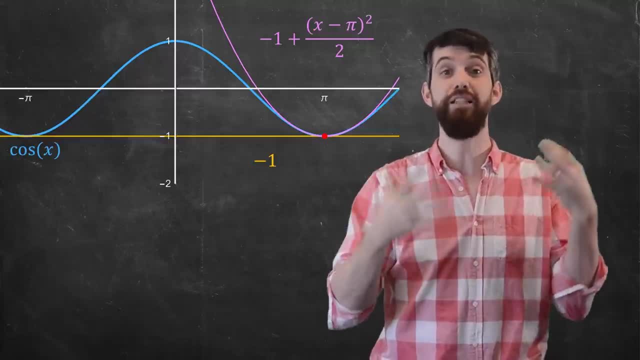 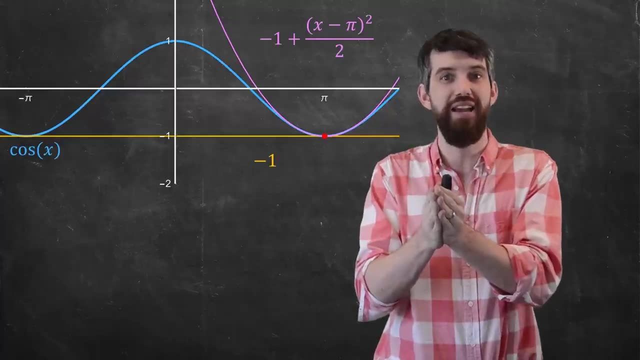 pretty good. Indeed, my polynomial has an x minus pi squared in it. This is centered at the value of pi. So Taylor series takes information at a point of specific a and gives you information nearby that particular value of a. It gives you local information.